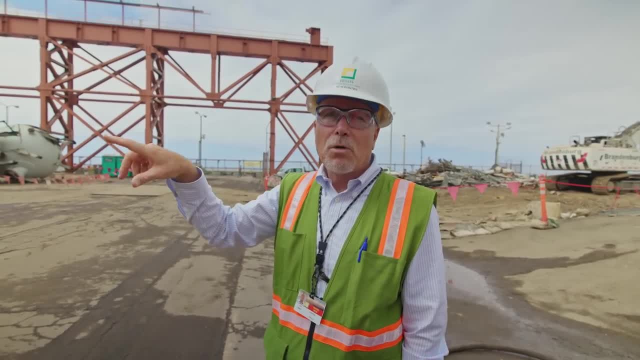 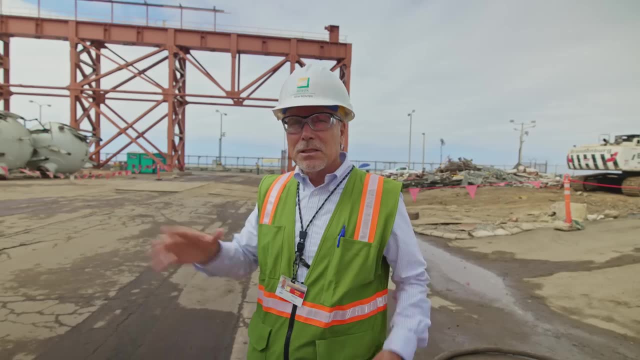 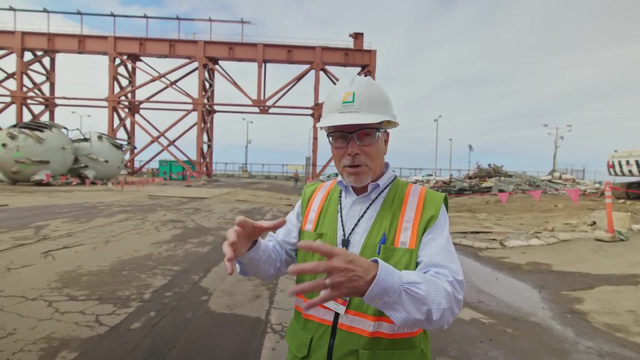 And that's basically a closed loop. It continues while we operate the plant and make electricity. okay, The plant would operate on a cycle of about 18 months of running continuously at 100% power. Then we would shut down the plant, dismantle the reactor enough to remove the fuel. 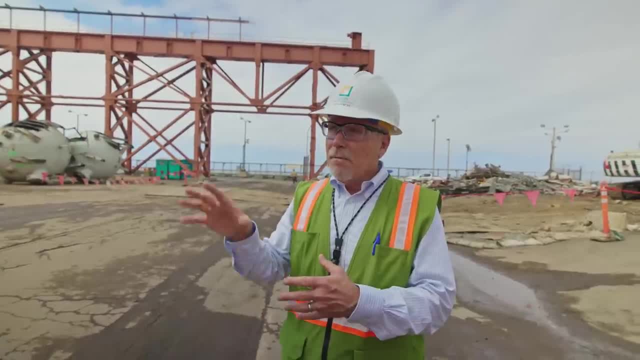 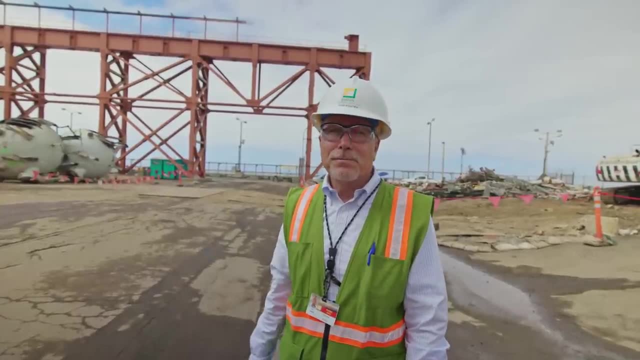 replace some of the fuel assemblies and then you know, restore the reactor, heat it back up again and start over and run for another 18 months or so. So now, how long would the refueling process take On this plant? it took about two months to go through the whole process. 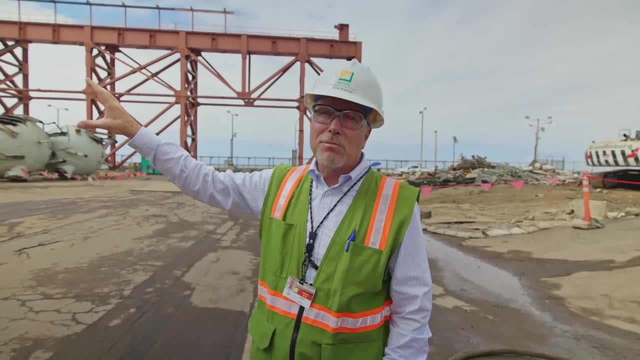 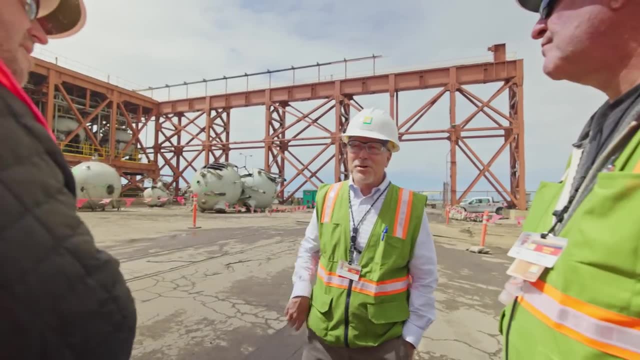 And while we were refueling a reactor, we'd be on this side of the plant doing maintenance on a turbine and other systems as well. Today, I think there's probably involved for all our operations probably about 400 people, 150, something like that. 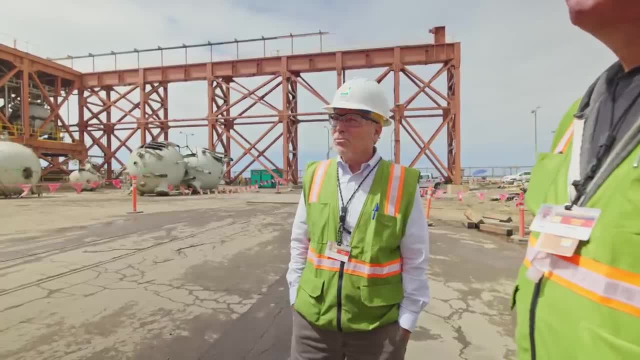 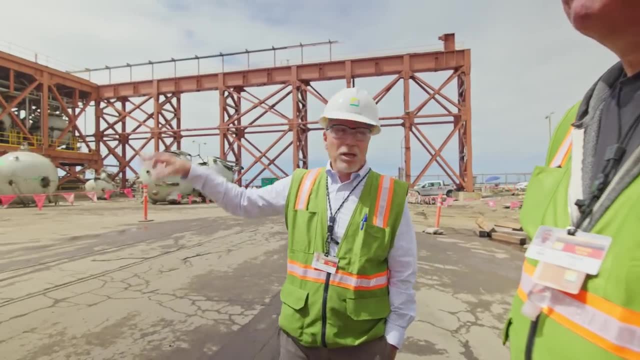 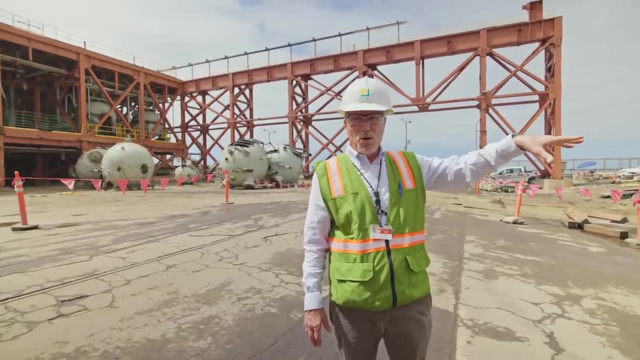 It varies day to day. So this was a pressurized water reactor. The San Onofre plant was a pressurized water reactor. This is Units 2 and 3.. Over there used to be Unit 1.. We started developing this site in 1964.. 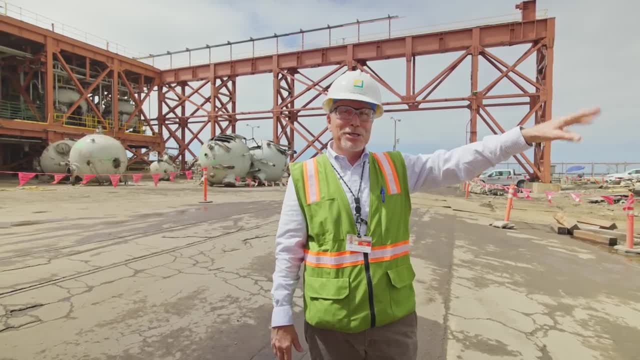 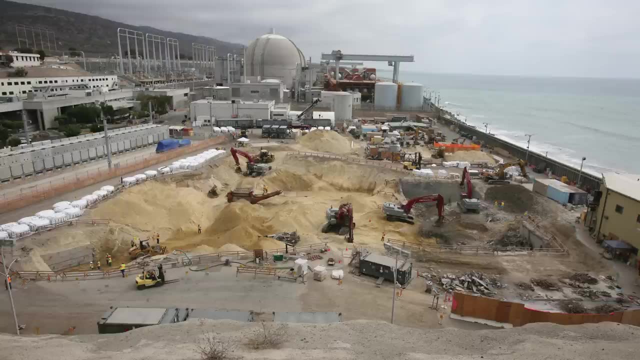 Built Unit 1, operated it until 1992, shut it down and then we dismantled it, mostly in the early 2000s, And in its place we built dry storage, A storage facility for the storage of spent nuclear fuel. So that's what exists on that location Over here. starting in the mid-1970s, we started developing this site to construct Units 2 and 3. And these sites were built together and came out of the ground together here And they went operational in 82,, 83, 83, 84 timeframe. I forget the exact dates, And they operated until 2012.. In 2012,, we had some issues with the new steam engine, Some generators we installed here And, after some consideration for about a year and a half, we decided the most economical thing we could do would be to shut the plant down. 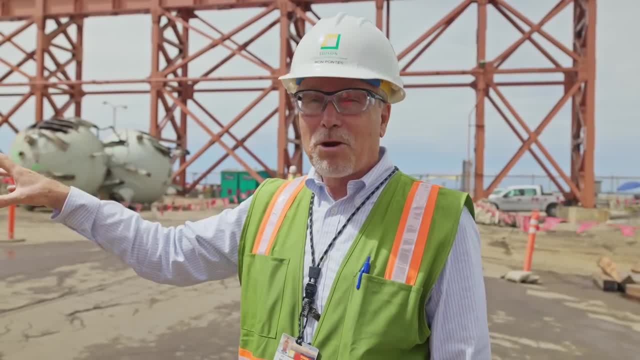 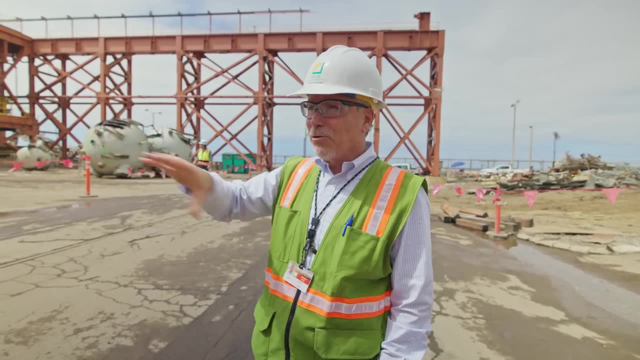 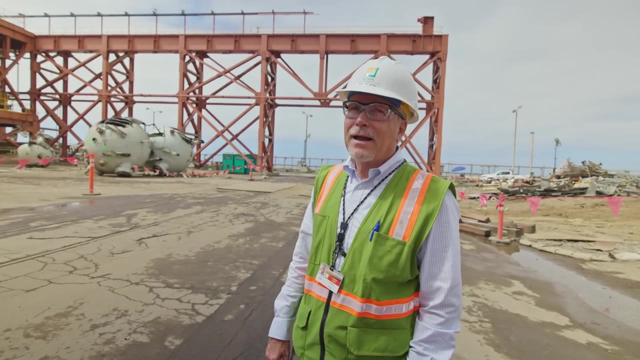 and move into decommissioning. So that brought us to where we are today. We started this active dismantlement work in 2020 after we went through a very rigorous environmental review with the State of California. So that was with the State of California, not the NRC. 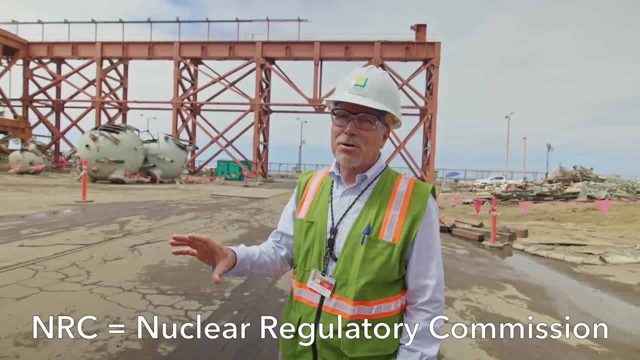 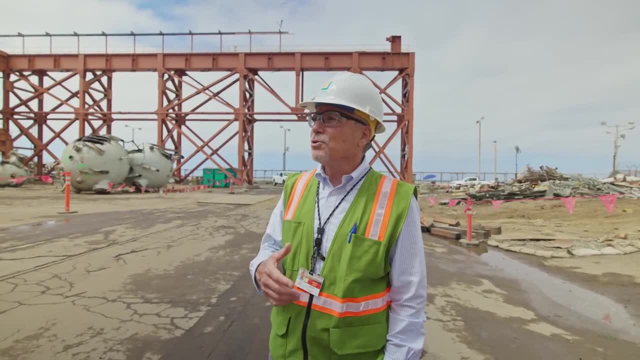 No, the NRC. we already had the approvals we needed from the NRC to start, But we needed approvals from the state- California Coastal Commission, California State Lands Commission. We needed their reviews and approvals And we finally got through all of that and finished with it in 2019.. 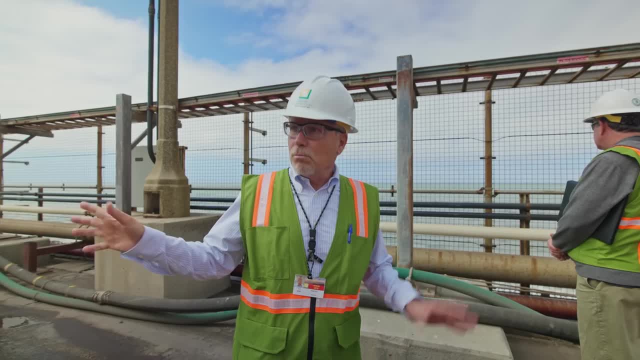 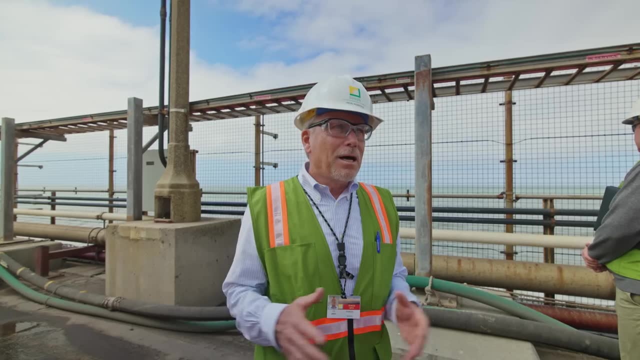 And then we started the real work in 2020.. The plant's built on Marine Corps Base Camp Pendleton. Edison leases this property from the Navy for the purpose to operate nuclear plants here. So you know we're in the process of dismantling the plant. then restoring this site to a condition that's going to be acceptable to the Navy, to take the site again. when we're finished here, The United States government's responsibility is to come, take the fuel, find a repository for it and then take the fuel from all nuclear plants. 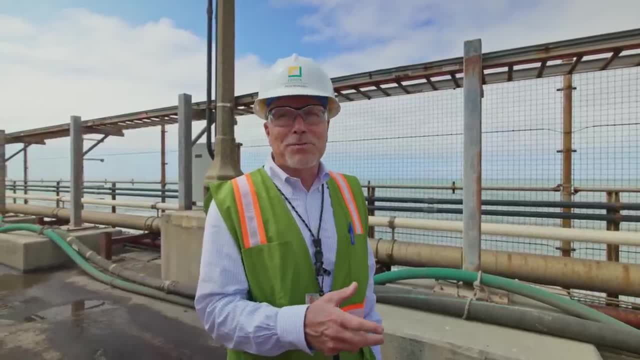 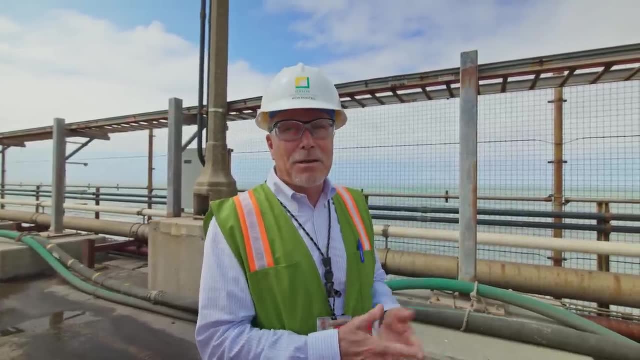 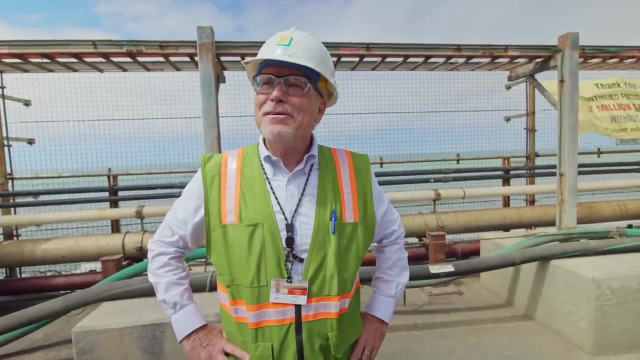 And so far they've failed on their responsibility. So until they figure that out, the fuel's kind of stranded here, like it is at all commercial nuclear plants. The non-radiological parts are all easy compared to everything else, right. Everything has its difficulties. 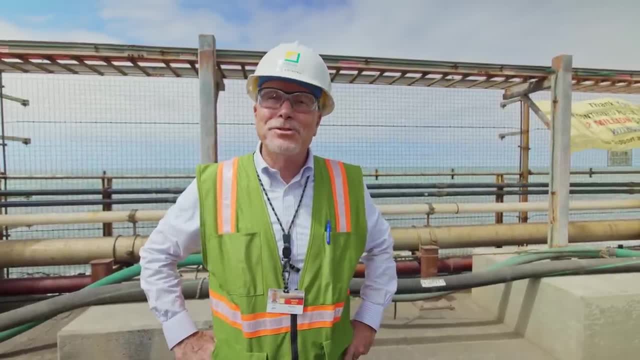 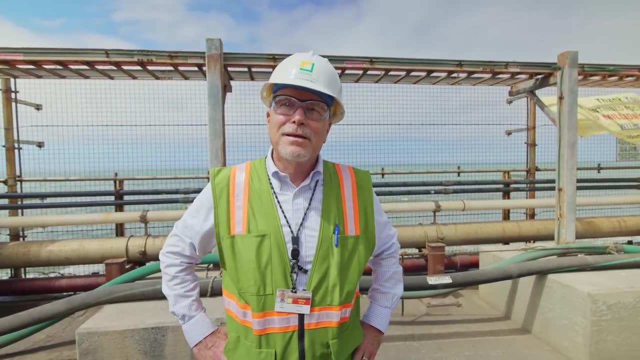 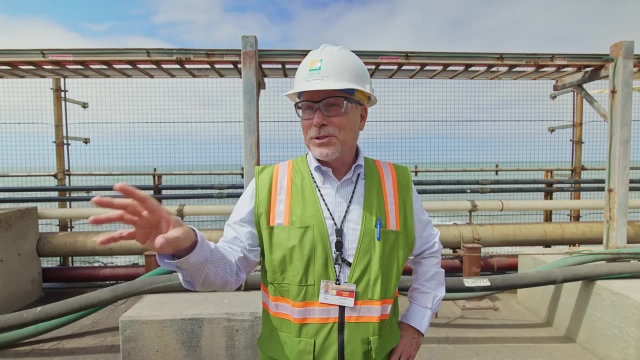 I wouldn't say. the radiological side's any more difficult. Some different methods are employed to control contamination and so on, And what are usually the contaminants you have to deal with in that environment? Actually, this is a very clean plant compared to some nuclear plants. 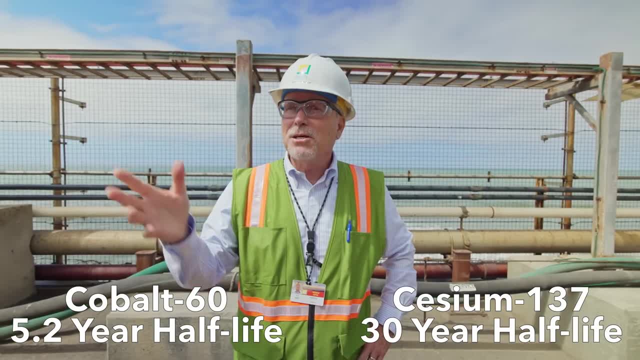 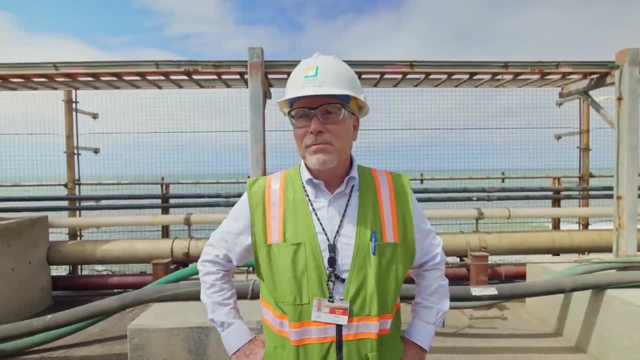 Mainly Cobalt-60.. Some cesium. Those would be the things, from a radiological point of view, that we would be most concerned with controlling the contamination, And that's all just from neutron. activation of the metals: Well, activation of materials, you know contaminated. 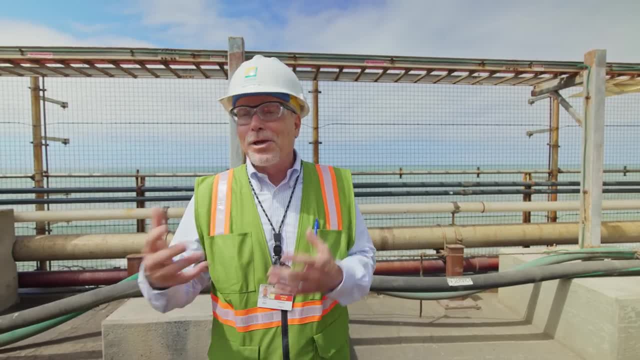 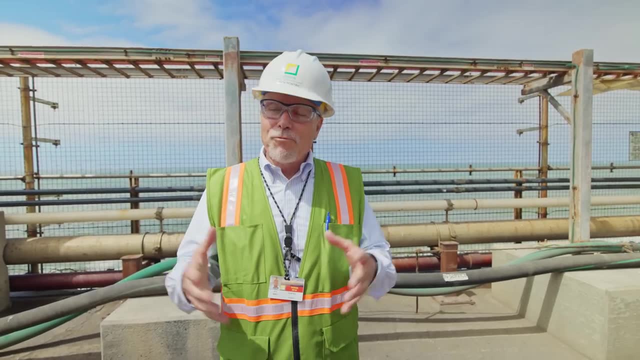 basically metals that are, you know, in the plant. Okay, You know corrosion products, for example, is where most of where the Cobalt-60 comes from. So you have wear of pumps and valves and that wear has you know. 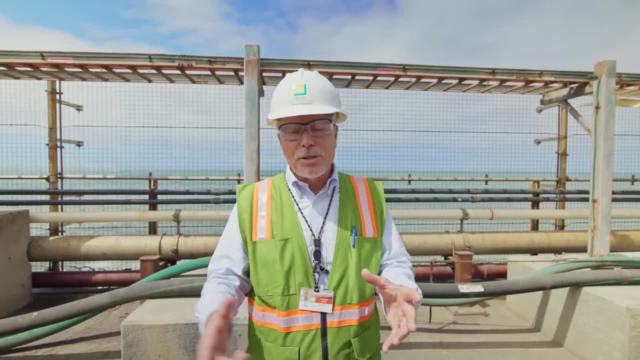 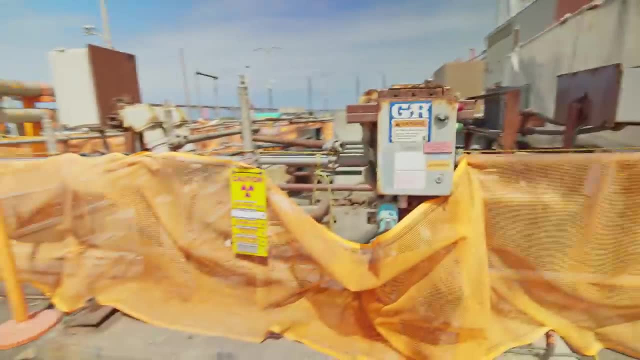 it has Cobalt in it. The Cobalt gets in the nuclear steam supply system. It becomes activated. That's where the Cobalt's coming from. So now, what's this? why would this be radiological Like? why do they have tags on them? 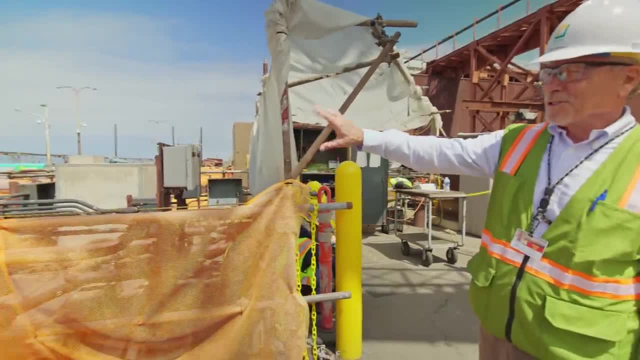 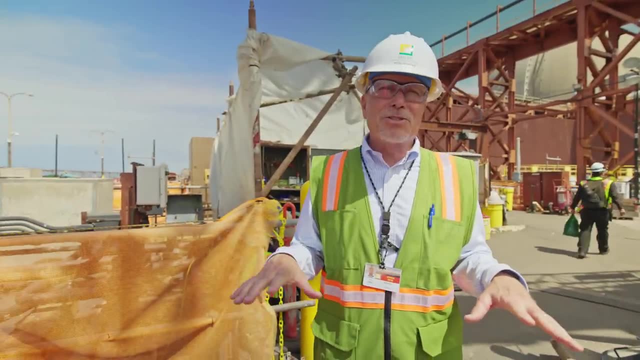 It's really just potentially contaminated. Just out of abundance of caution, we got a tag like this: Okay, This is just part of the. this is where we're standing is part of the intake structure. Okay, So we drew when we were operating the plant. 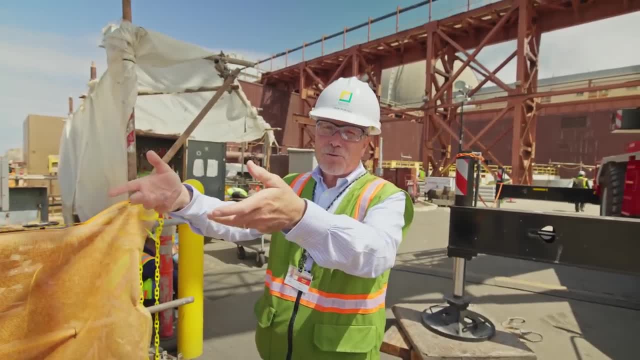 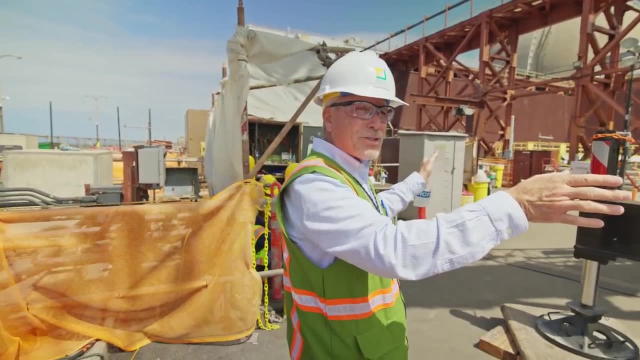 we drew water in from the ocean from the conduits that are installed offshore. That water flowed in here and then went to Unit 3 or Unit 2 to cool the condensers, and then it was discharged back to the ocean. 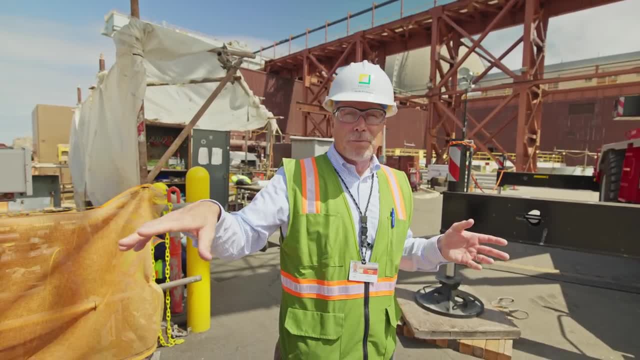 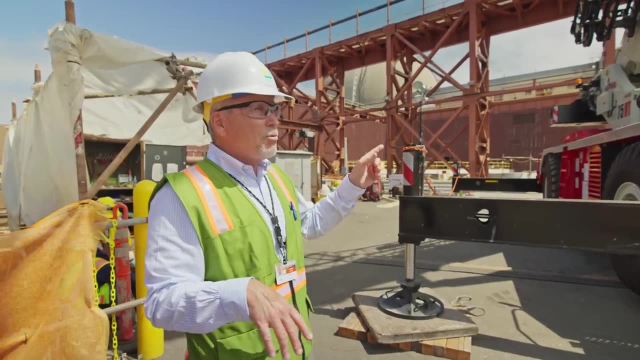 So that was basically an open loop to the ocean. Okay, Okay, So that was its whole. purpose was to cool the condenser Now, so you know, the plant generated about 1,150 megawatts when we were electrical power. 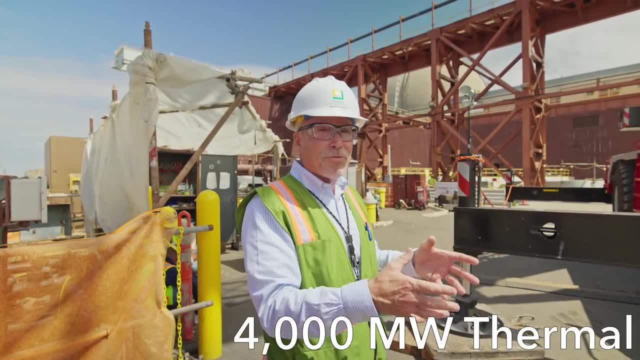 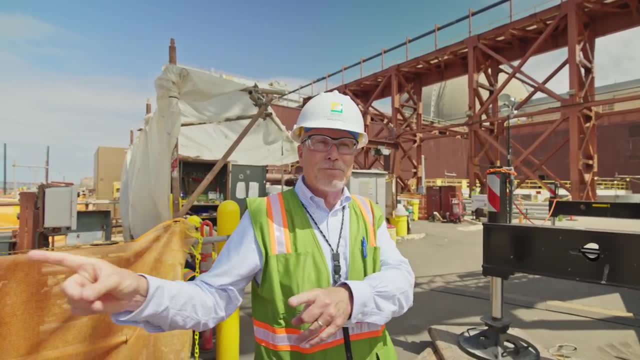 But to create 1,150 megawatts, that's about 4,000 megawatts of thermal energy. So it turns out that, unlike all these plants, most of the energy ends up going to the ocean, the heat sink. 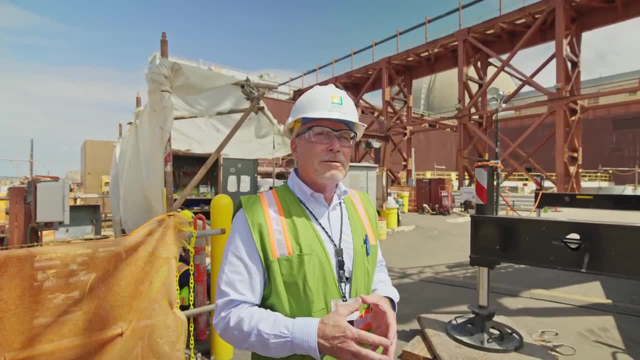 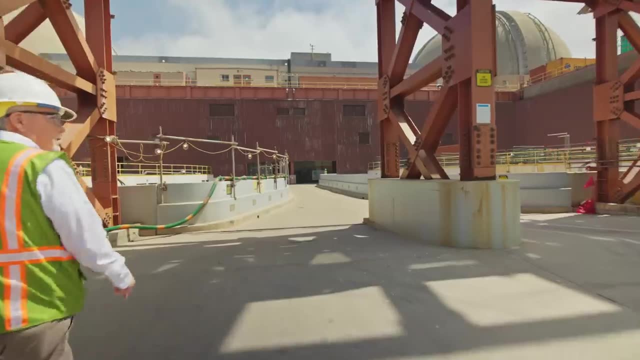 because they're only about 32, 33% efficient. Wow, Okay That's. if you had an oil-fired plant, it'd be the same, or a coal-fired plant, it'd be about the same efficiency. So we no longer bring water into the plant to cool it. 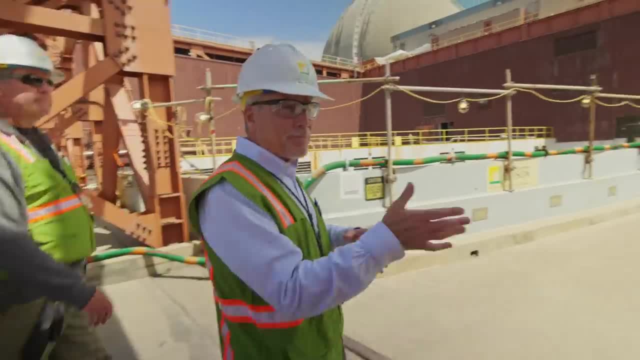 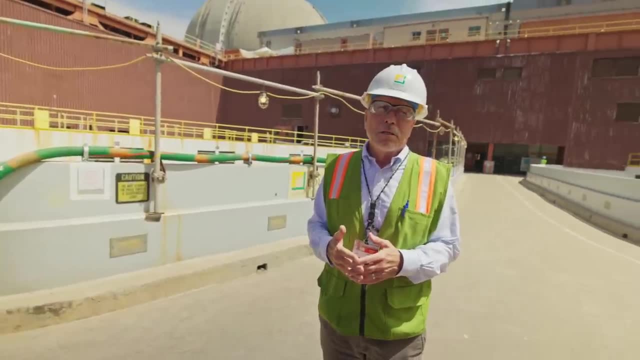 We don't reject any heat. now to the ocean. All this system is isolated. You know how much heat actually was it like that would come like from the plant back into the ocean. So there was a small temperature rise in the water. 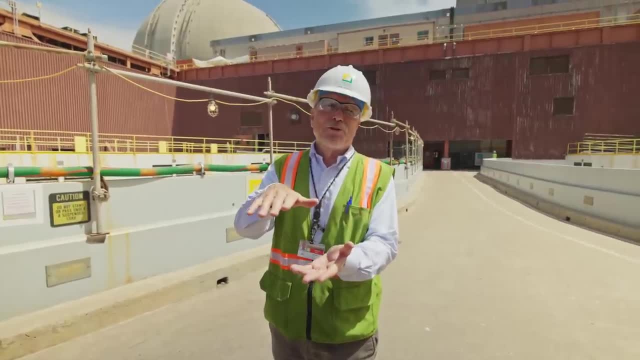 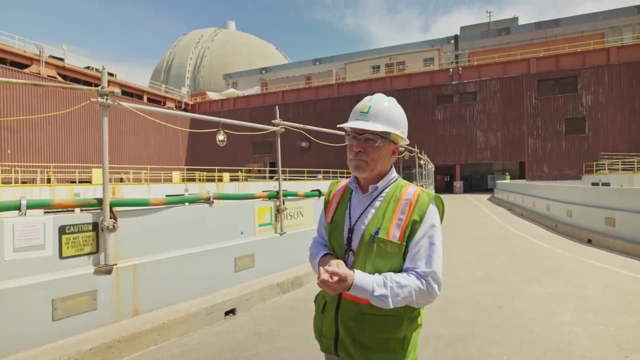 that we deposited back in the ocean just a couple of degrees. Oh wow, that's not bad at all, Because it was distributed through a bunch of diffusers on these conduits. Okay, Okay, Processing about 1 million gallons per minute per unit. 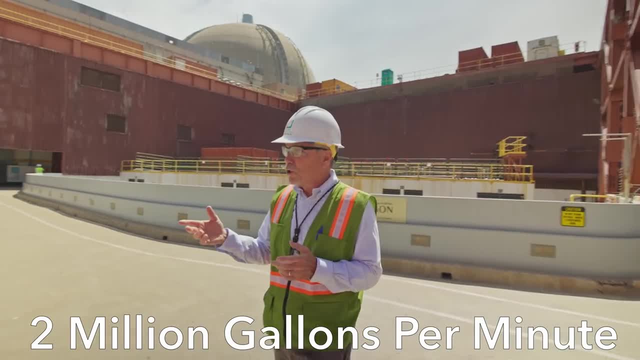 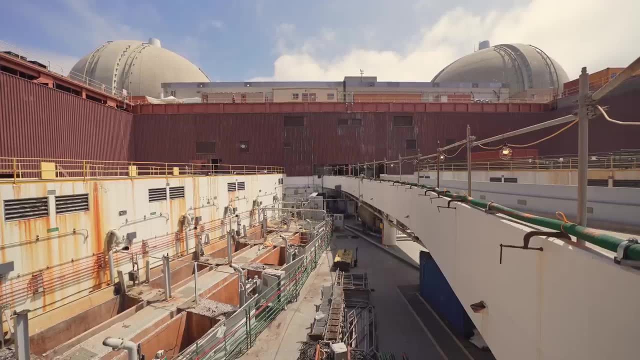 when we were operating. Wow, So about a lot of water. There were huge pumps that were installed here or just beyond those walls. There were big circulating pumps that were used to move the water from the ocean through the condenser and then back to the ocean. 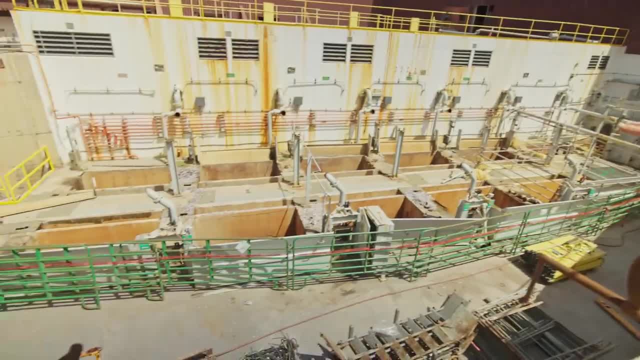 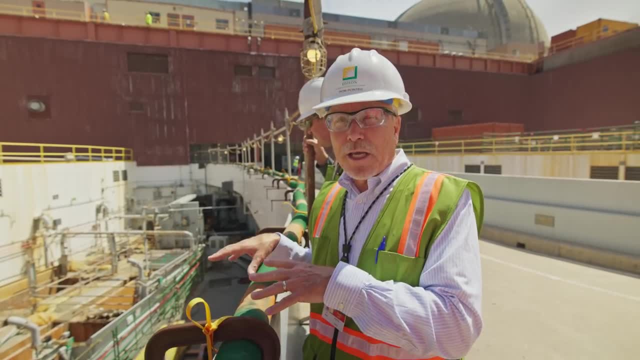 In this area. it's been removed now, but in this area is where the traveling screens were to take out any debris that was in the ocean water, like seaweed for example. We also entrained some fish right. Those fish would collect there unharmed. 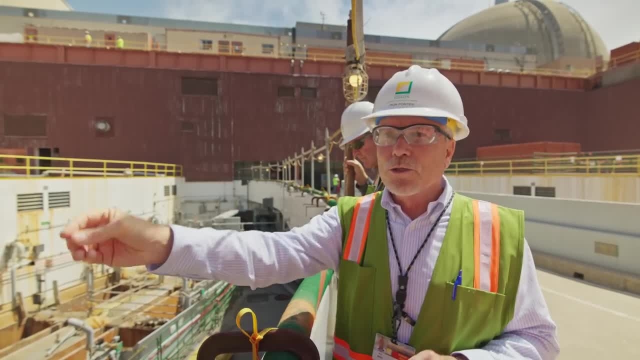 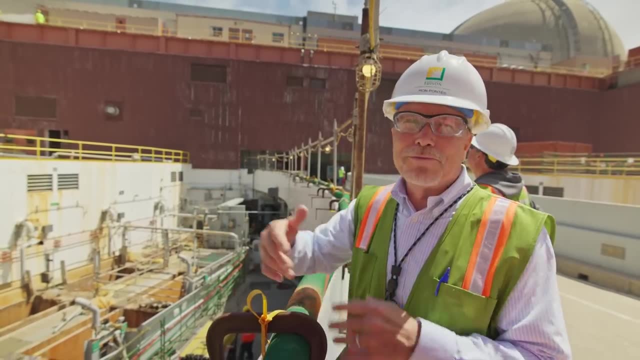 and this elevator would lift them and sluice them back to the ocean through another conduit. Wow, And that's continuously happening, right? So any fish turned to the ocean basically unharmed. Now also, sometimes marine mammals would come in. 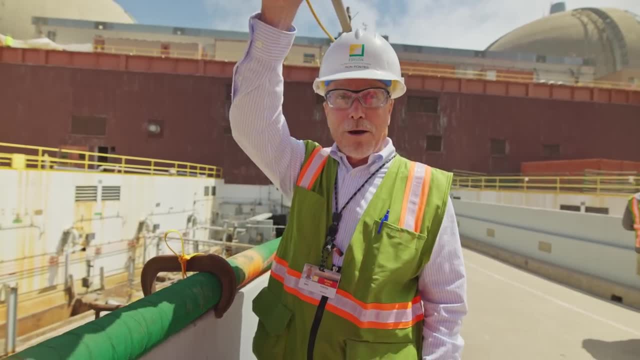 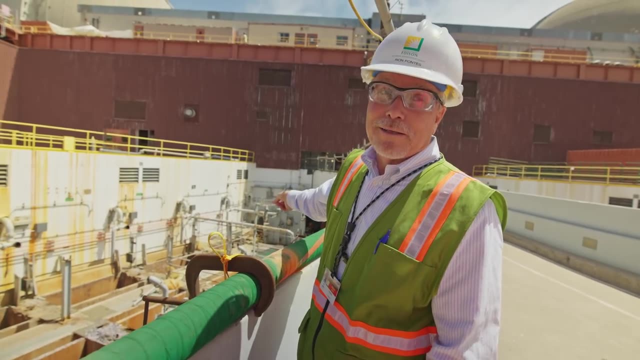 like sea lions. Wow, They would enter the conduits way offshore, take a ride down here and end up right over there. Oh man, And it was like a smorgasbord, right? Not a bit, Right. 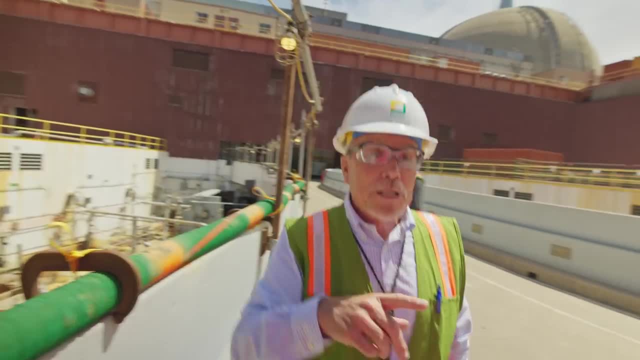 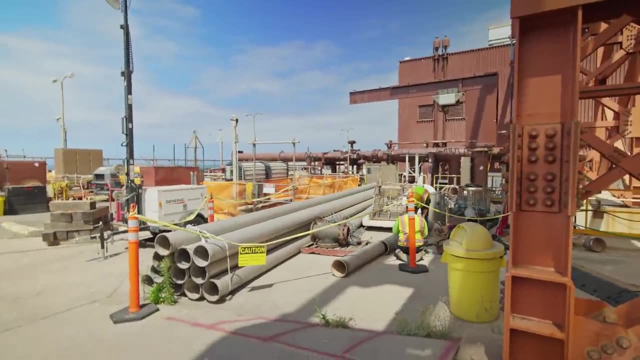 So they would be consuming fish. Well, one learned about that and they're like, hey, we're going to go to the center, They would come back, We would capture them. You see that cage? Yeah, Okay, So we would collect the marine mammals. 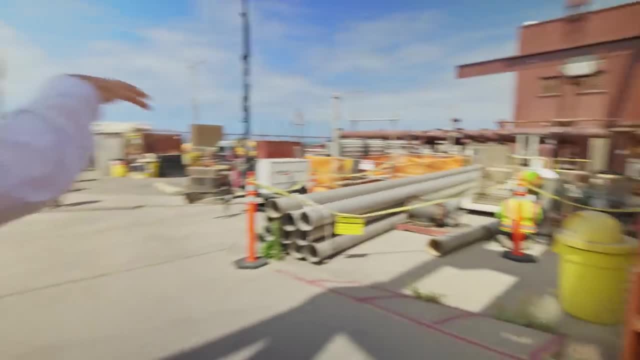 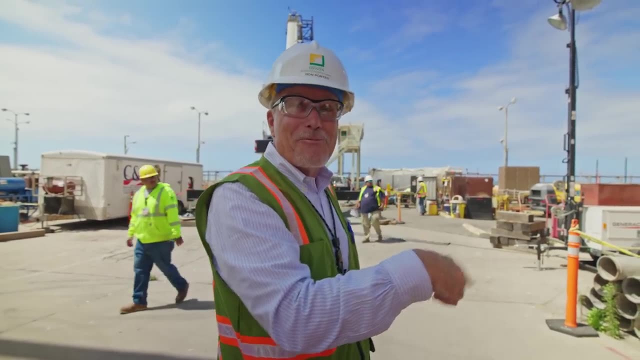 when they did arrive here in these cages and then take them on a truck and put them back in the ocean someplace right- And sometimes they would return, You know they'd find their way back. So now everything below ground is going to be backfilled with concrete, right. 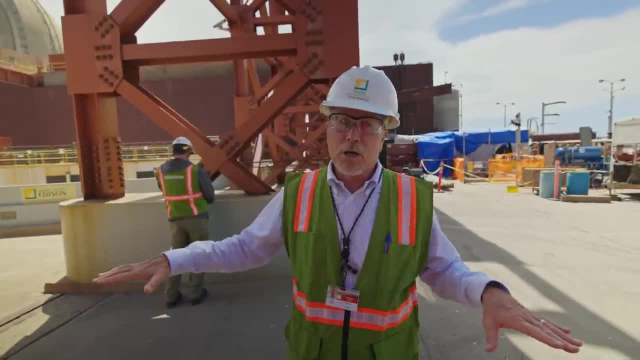 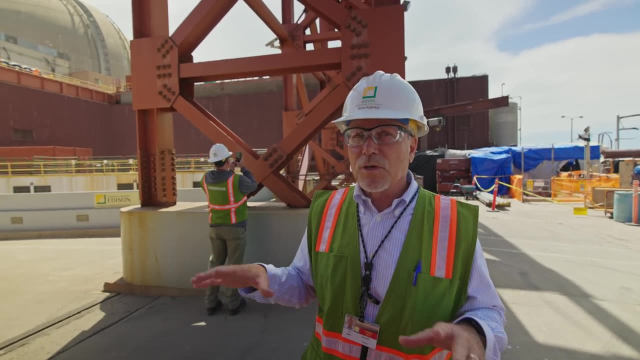 Not with concrete In this area. we're going to fill this area with concrete because we need a good, solid surface to work off of. But the rest of the voids that are remaining after we complete this phase of decaying commissioning. 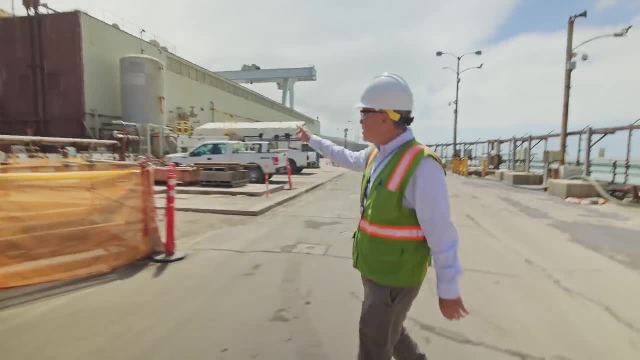 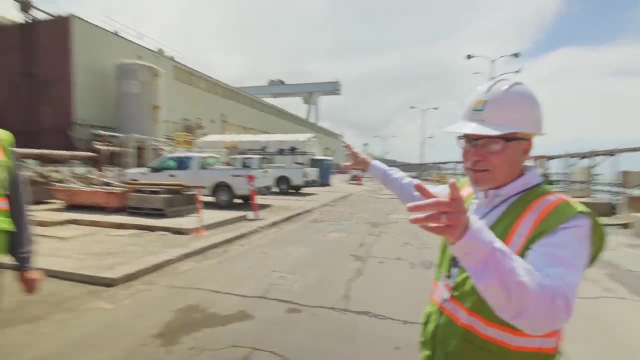 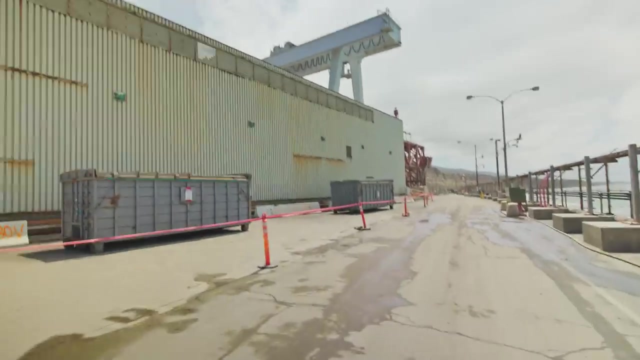 will be backfilled with native soils from here on site. So, Drew, this is the Unit 3 turbine building. You can see this part of it's largely intact. That's what Unit 2 looked like just a few weeks ago. So now, with these cranes, 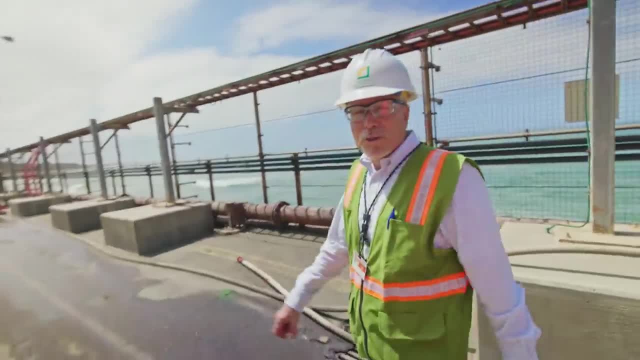 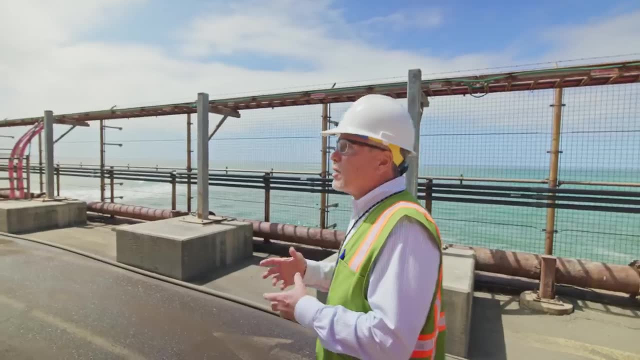 what were these primarily used for? To service the turbine generator, for maintenance the turbine rotors and the generator itself. So when we would shut down for the refueling outages, we would dismantle, you know, parts of the turbine, the generator, inspect and then restore it. 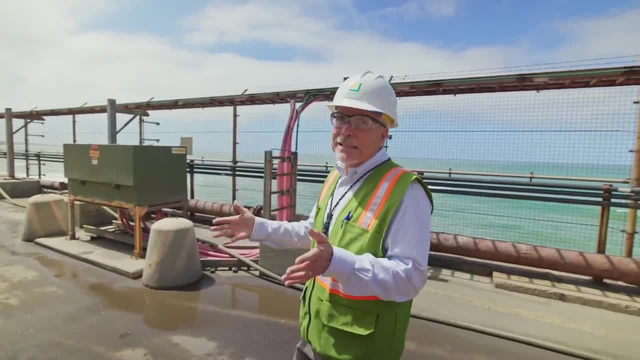 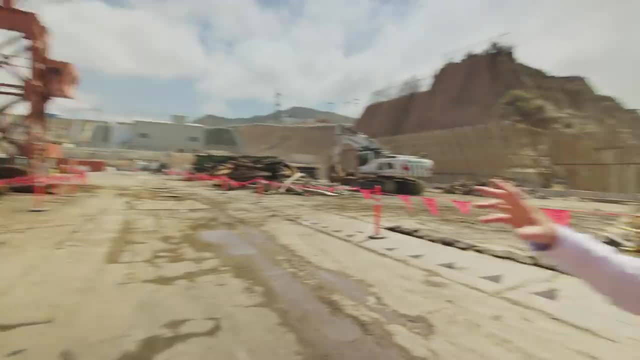 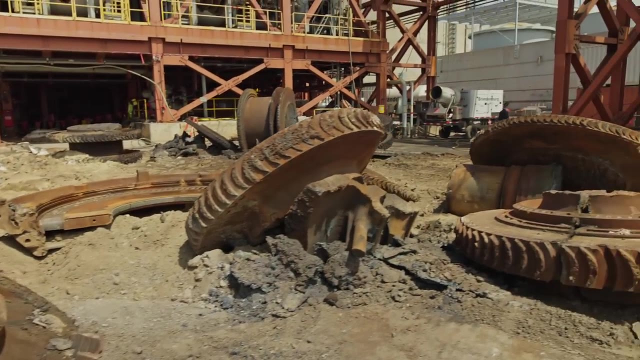 Because you know we wanted it to operate reliably for like 18 months continuously. These are remnants here of the Unit 3 turbine rotors. The contractor's been cutting these up into manageable pieces. You see how big those components are. They're huge right. 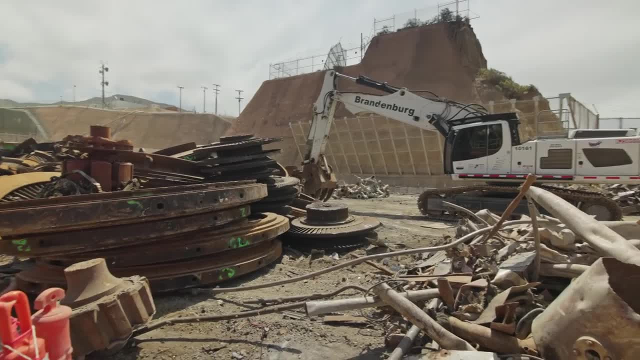 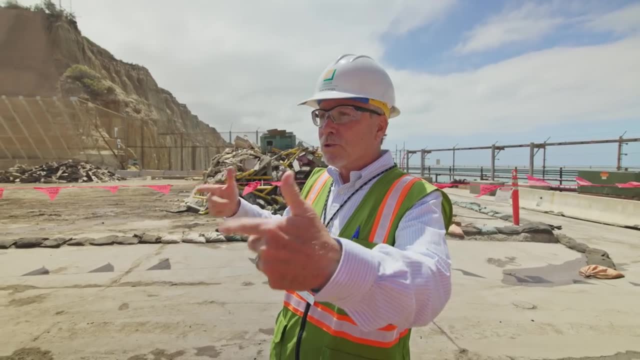 At one time. you see all this scrap over here. They were basically turbines right With different stages And they were like huge wheels that would spin when steam was admitted to them, And you can just see what's remaining here of all of this steel. 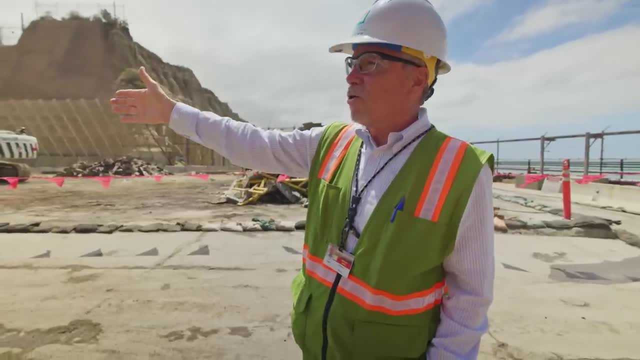 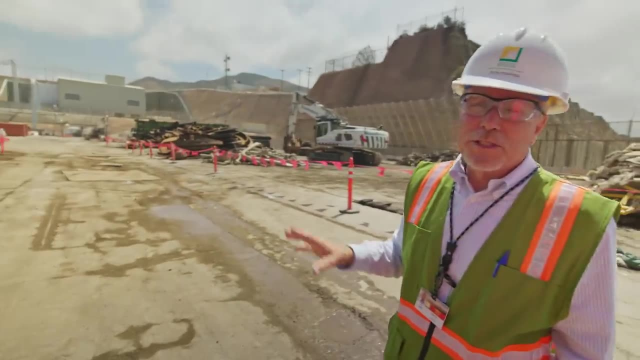 So, again, all this stuff, it gets chopped up into smaller pieces and then it's going to be sent off site to be recycled. So it's just primarily steel, Just steel, yeah, Carbon steel. So this is what's left of the turbine. 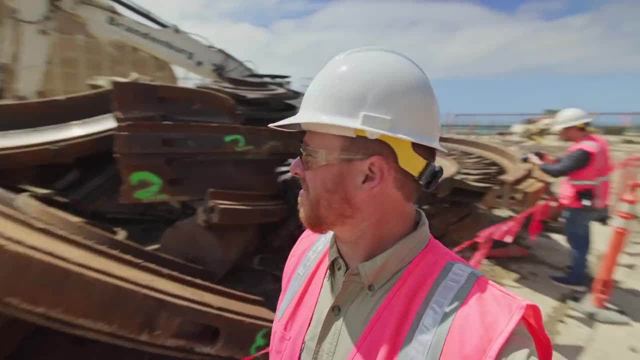 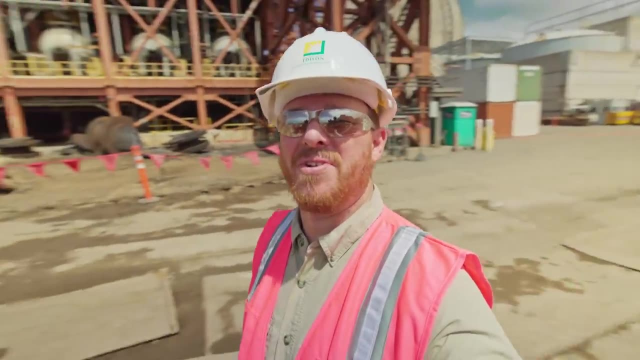 It's been cut. It's been cut up pretty good And it is massive. There's a lot of material here, Kind of at a loss for words at how incredibly huge all this is, And it's not until you're like, really close up. 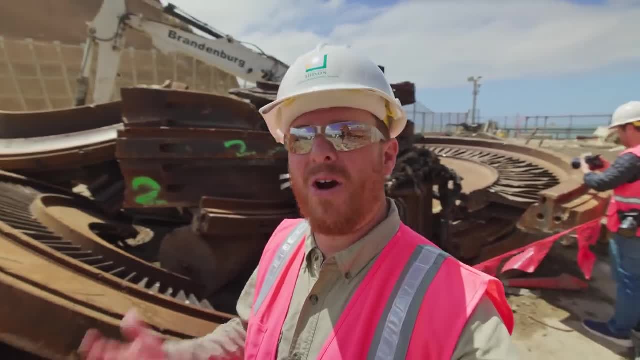 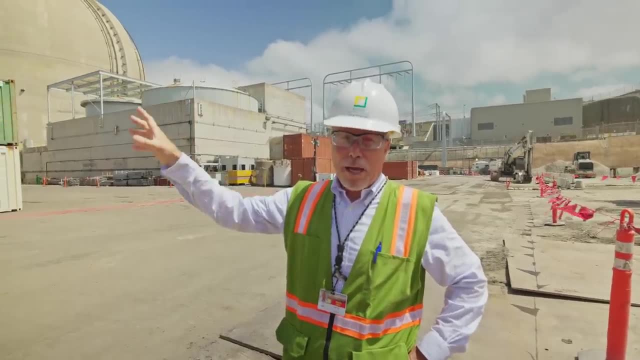 to something like this that you can actually understand the scope and size of a power plant like this and how much energy it produced. It's very impressive. The steam generator had to be reliable in its operation. For it to be reliable, it can't vibrate. 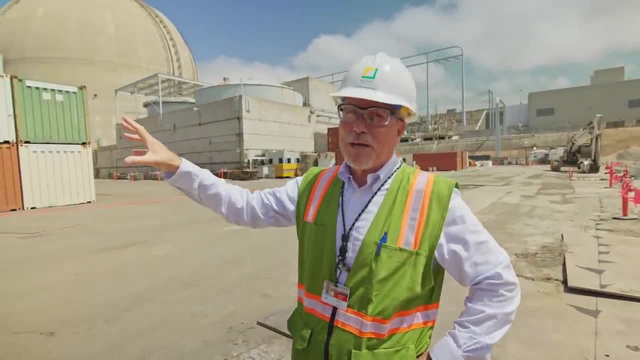 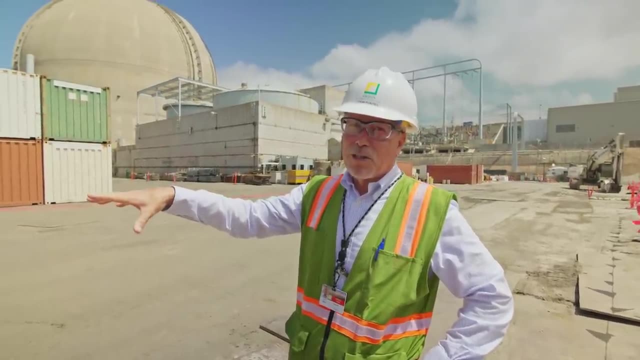 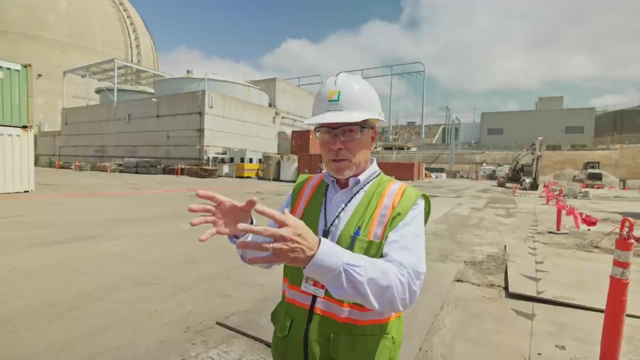 To make sure it doesn't vibrate. you need a substantial foundation for that machine. The bottom of the turbine building the foundation is 15 feet thick of reinforced concrete And on top of that foundation were built pedestals, basically columns that rose up from that foundation. 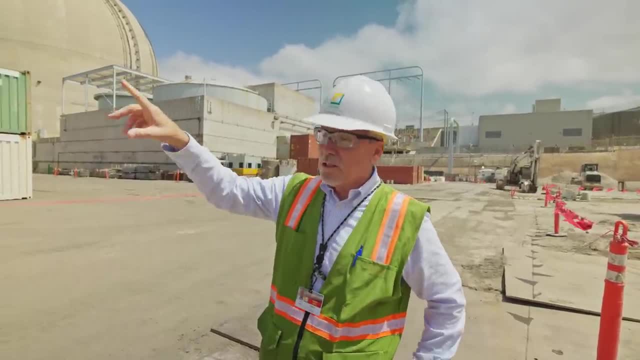 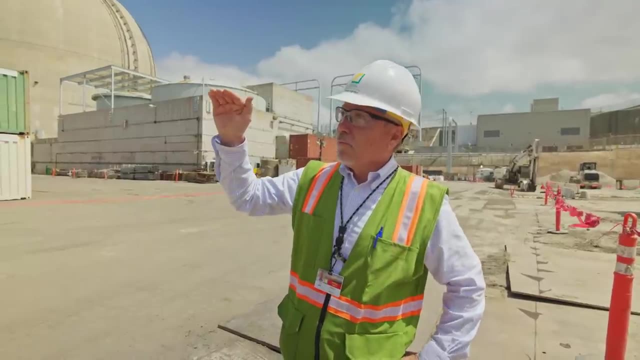 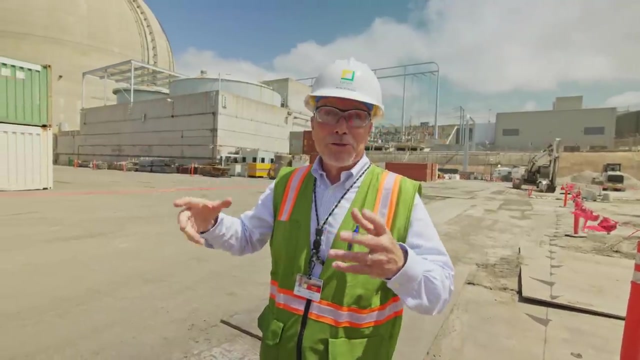 to support the turbine. The turbine was not supported off this steel. you see here It was supported independently off of these columns, or pedestals as we call them. So that created the foundation. so the turbine was reliable in its operation And it was a very well-balanced machine. 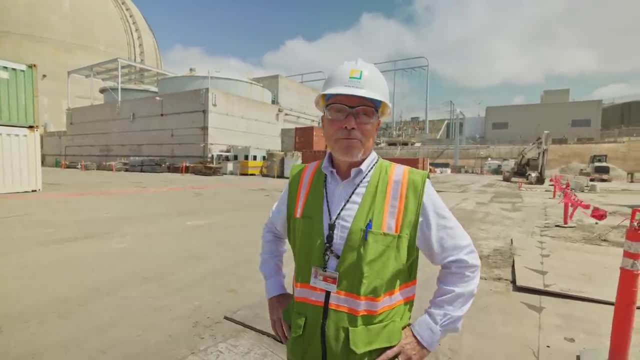 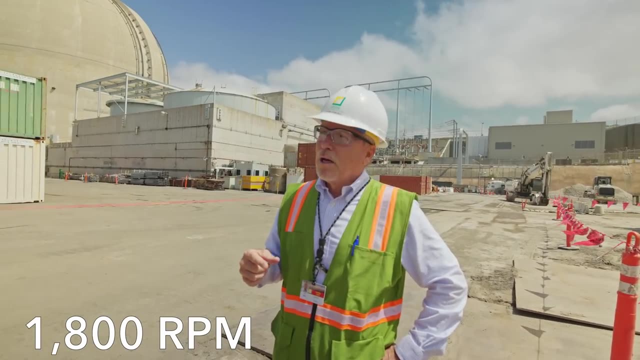 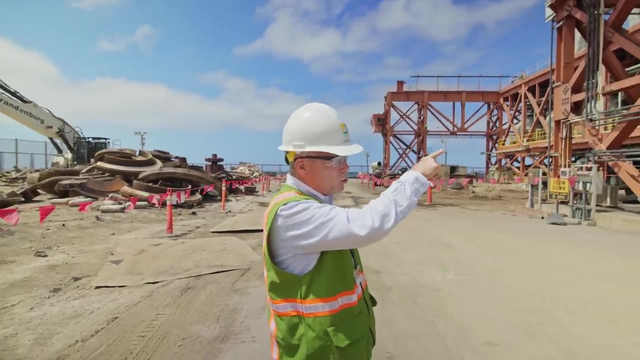 again, so it doesn't vibrate and operates reliably. for like an 18-month run It was rotating at 1,800 RPM and it was generating voltage at 24,000 volts, And the output of the turbine generator was connected here to a huge transformer. 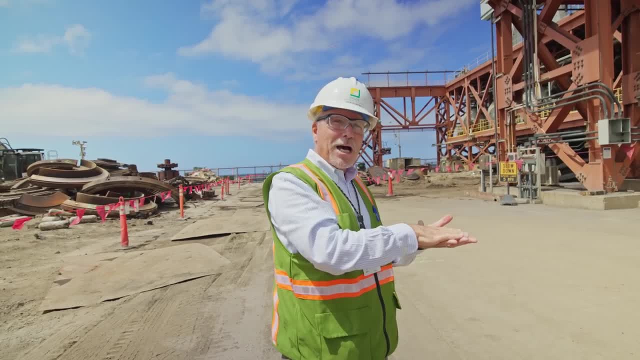 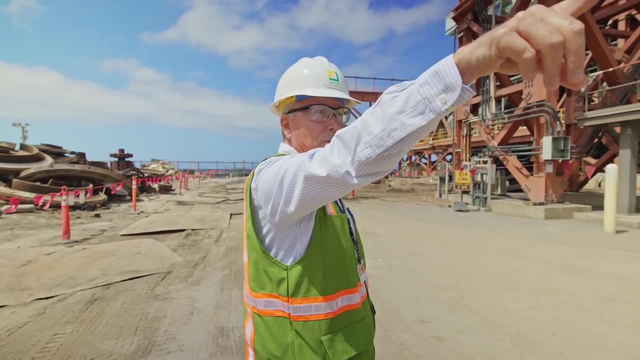 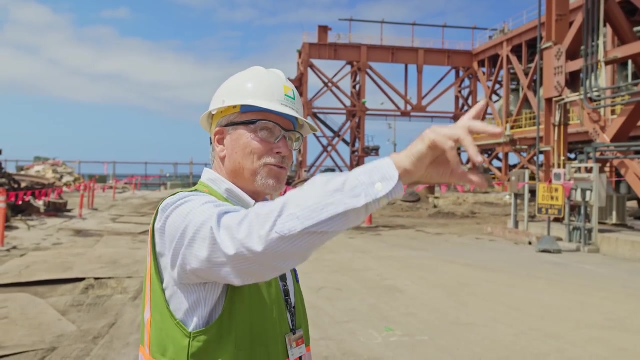 And that transformer would boost that voltage up to 220,000 volts. At one time there were power lines that connected from the switch yard here to that transformer. The voltage boosted here to the grid- voltage, 220,000 volts- is connected to the grid. 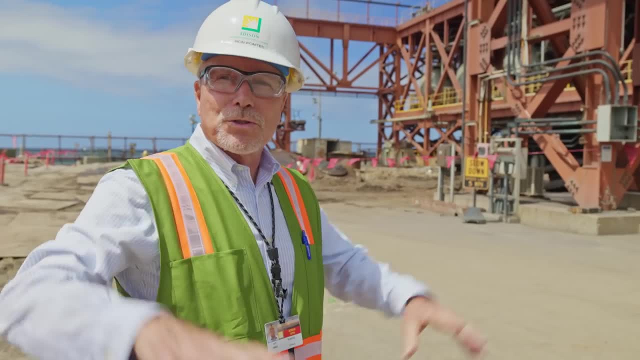 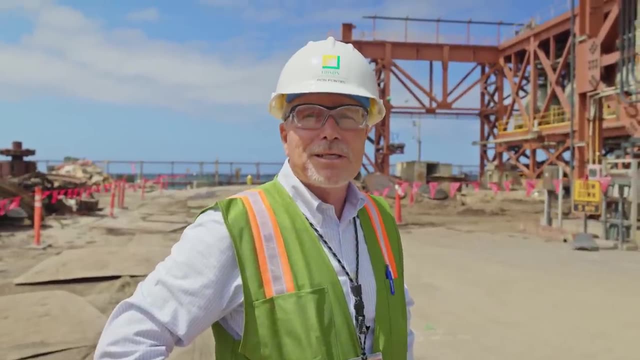 and then that's what was supplied to our customers, Of course, through a distribution network that reduced the voltage down to like what you use in your house- 120 volts or 220 volts like that. So this switch yard today is really just an interconnect. 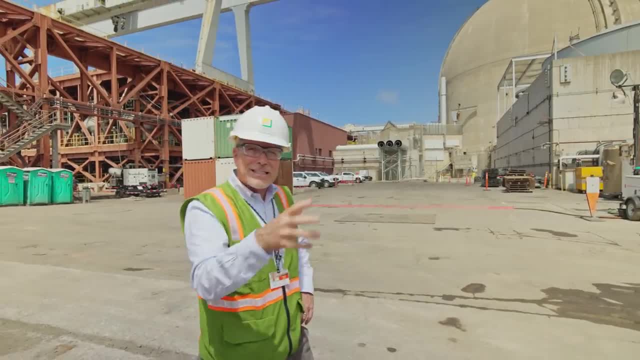 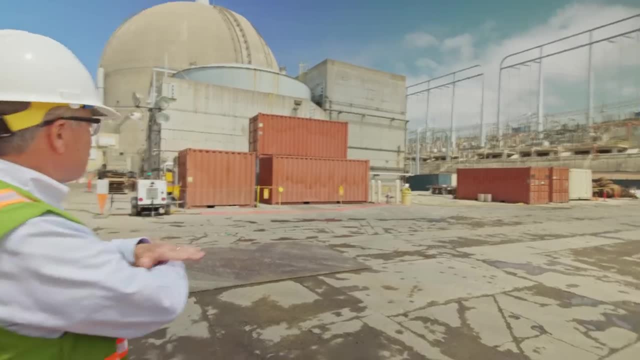 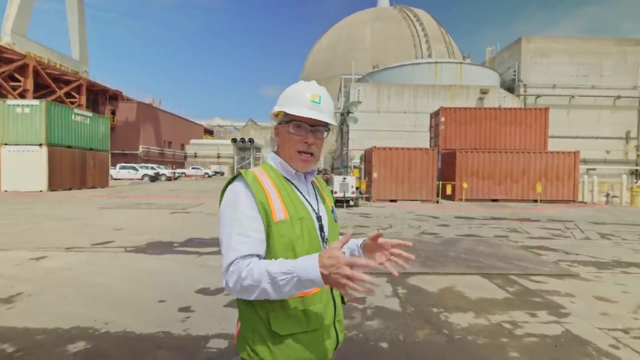 between Southern California Edison's transmission system and San Diego Gas and Electric's transmission system. They connect right here, So that's going to remain too. Everything else that you see here is removed to at least three feet below where we're standing. Then what remains is cleaned up. 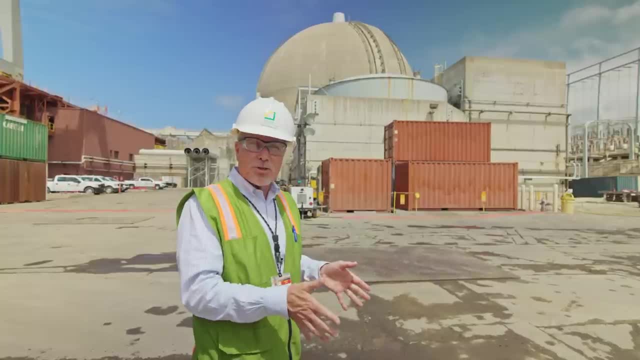 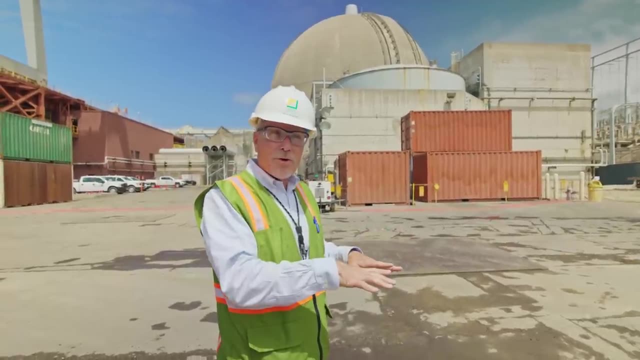 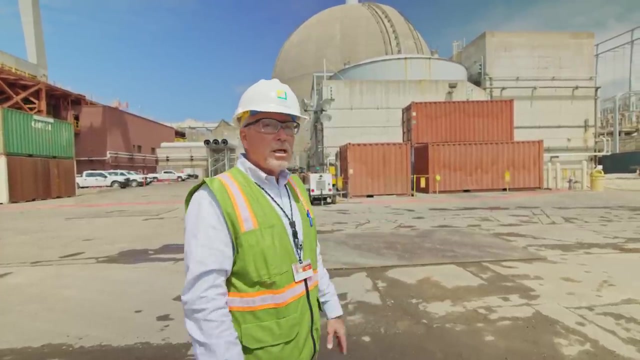 decontaminated to meet NRC license termination requirements. Then we're going to backfill everything. All the voids that we created will be backfilled with native soil And then we'll stabilize this area basically back at this elevation And we'll wait for the government. 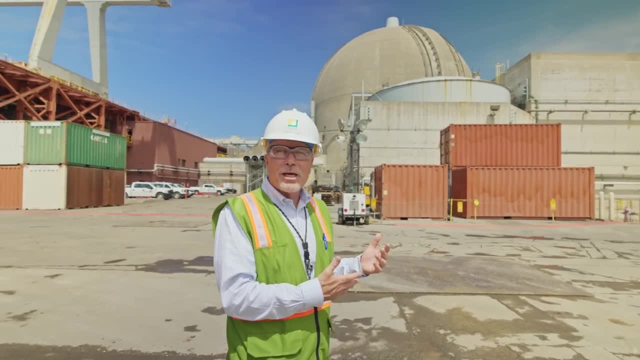 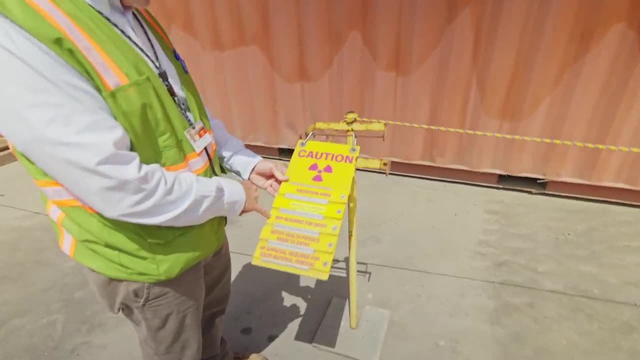 to do its job with the spent nuclear fuel. okay, to remove it from this site. Yeah, so this is a radiation area, radioactive material storage. You need a radiation exposure permit to go inside. You have to notify Health Physics before entry. 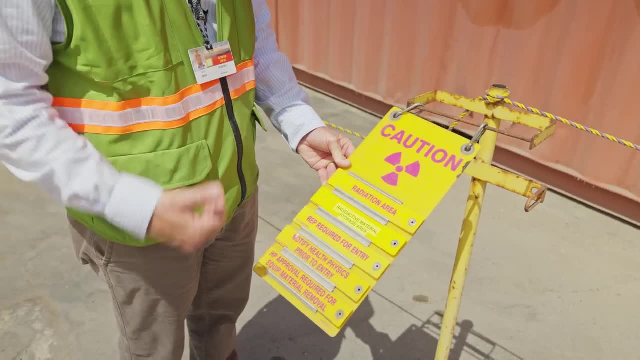 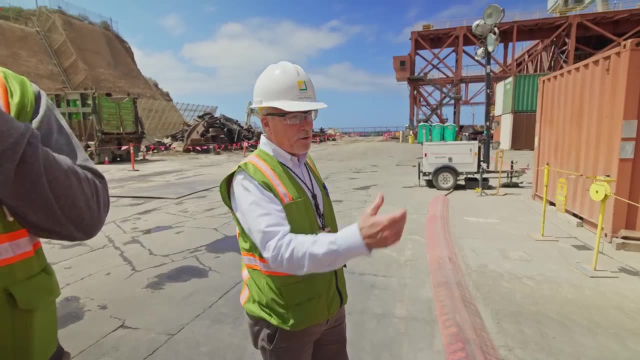 And you need Health Physics approval to remove any of this material. okay, So this is a typical sign that you might find for a radiation area here on site. This is a barrier beyond which, unless you meet these requirements, you're not supposed to go beyond that limit. 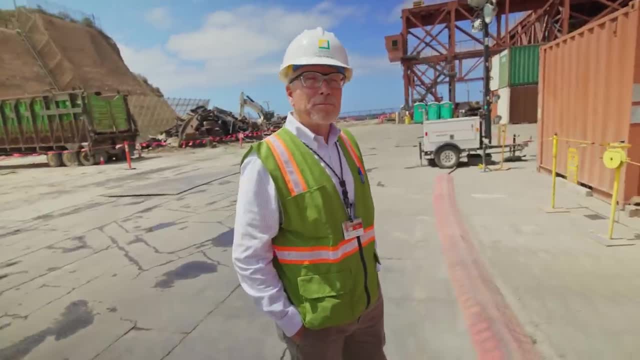 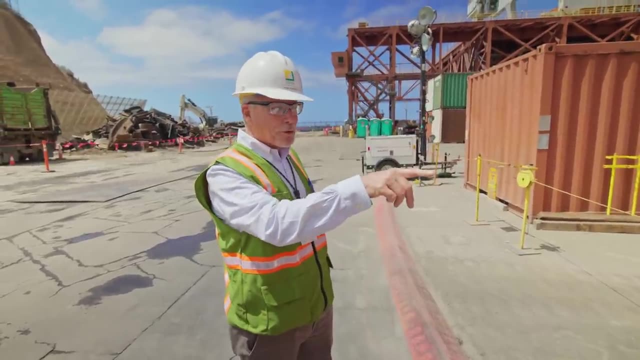 So you guys have different color rope. that signifies different things here on site. Yeah, this is yellow and magenta. It looks like the magenta's kind of faded out and the particular rope looks a bit more purple, but that's what this is, yeah. 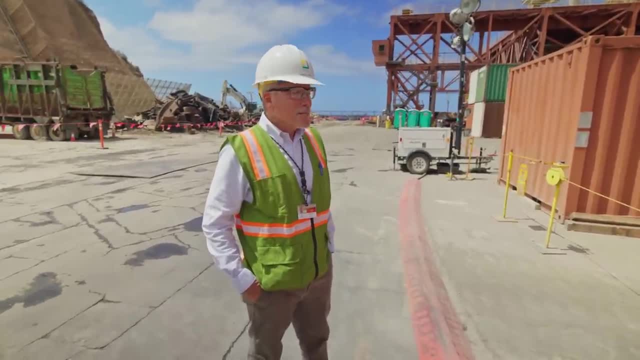 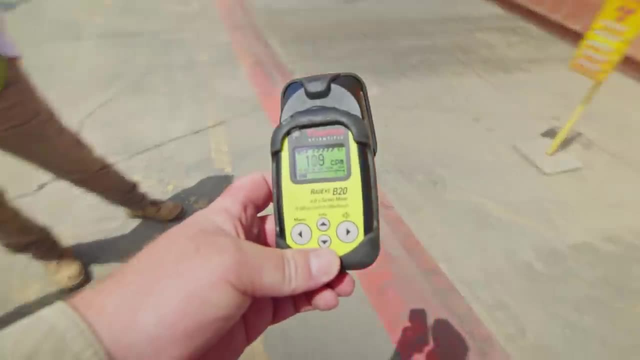 Okay, So this is supposed to be a glass wall. Yeah, It's like where you can look at it. you just can't cross it, You don't reach over it, Yeah, Or anything like that. yeah, Oh, there's definitely an increase here. 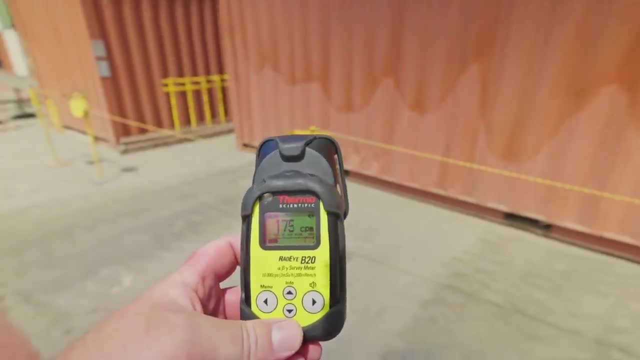 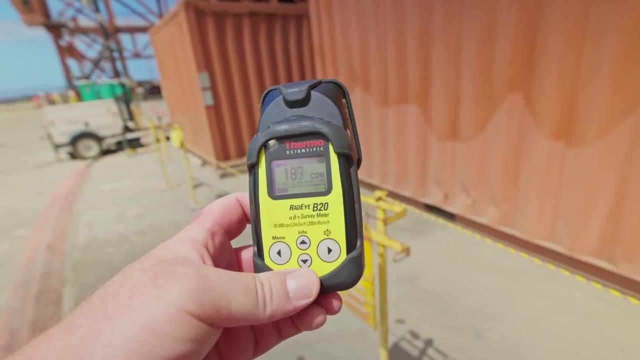 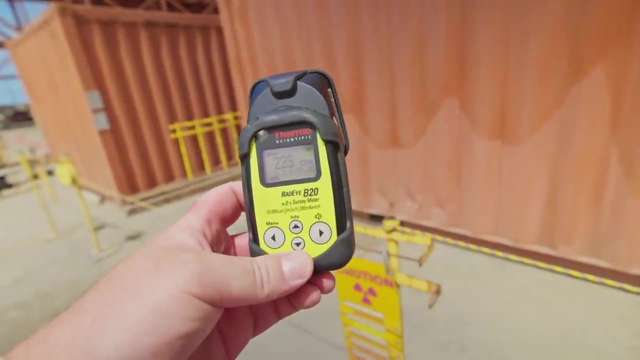 Not a lot, but Yeah, if you go right up to the, I mean it's barely anything. Yeah, It's like maybe, Eh, almost probably- like eight times above background. You know you were measuring count rate. 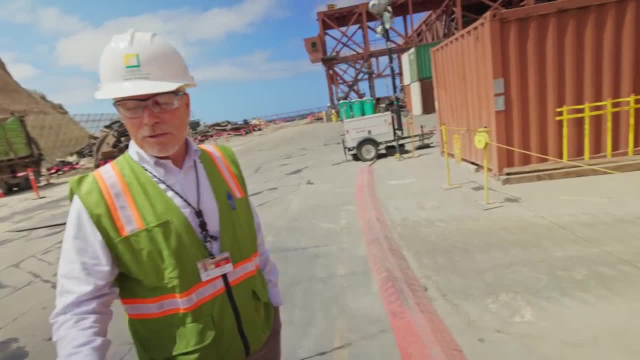 We usually didn't measure millirem. I know That's what we're using, So you know. later today Jeff will show you our meters and so on. Yeah, it was kind of cool with this one is I could actually switch it over to millirem. 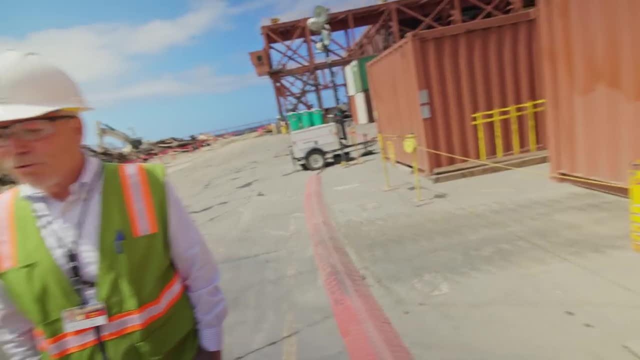 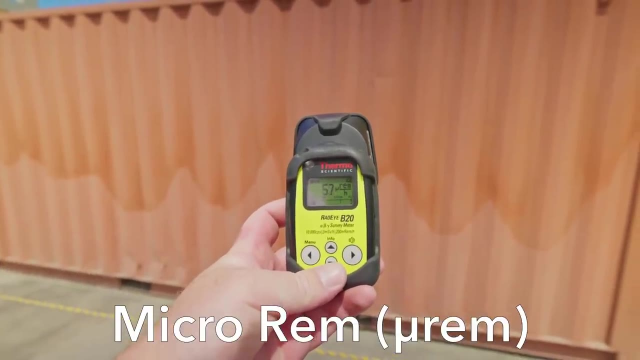 and to counts and sieverts and grays and disintegrations. What was the millirem? Huh, What was the millirem? Something 50. 50 micrograms, Yeah Yeah, 60. 60 micrograms. 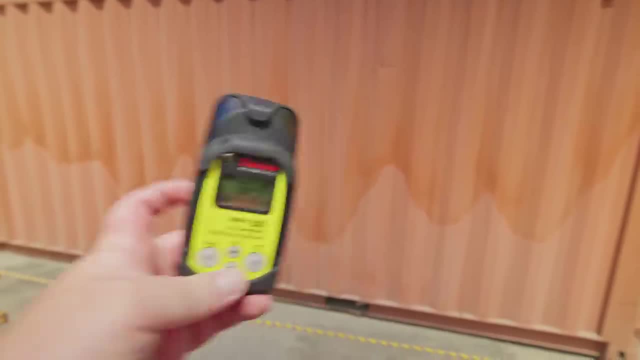 Yeah, so I don't have a filter on here. Pretty low, Yeah, Yeah, but still that's like: yeah, really really low Containment dome. That is a really substantial structure. It's an engineering marble actually, So it's about four feet thick. 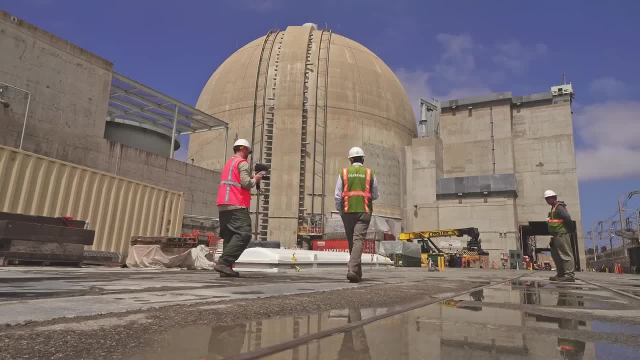 It's reinforced with steel And then, after it was constructed, it was tensioned. okay, We call this a post-containment. So it's a post-containment. So it's a post-containment, It's a post-containment. 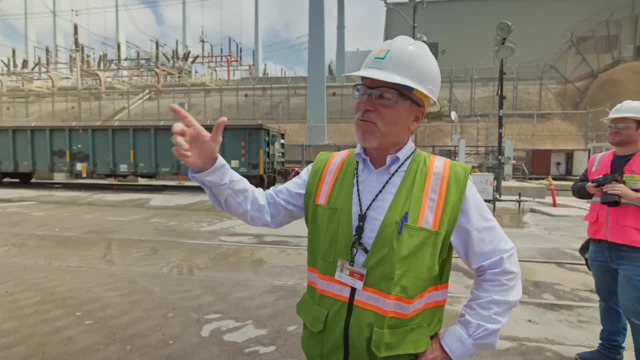 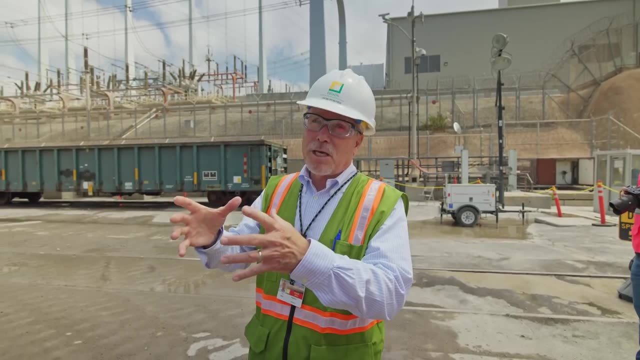 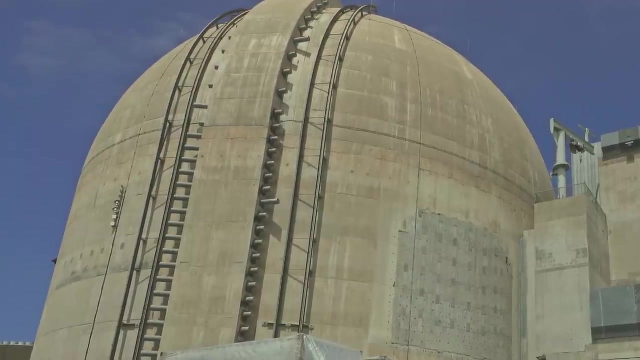 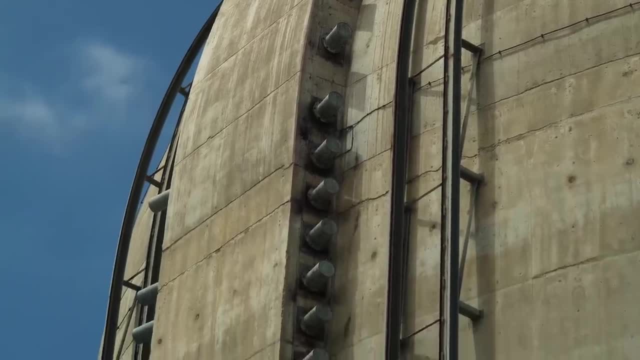 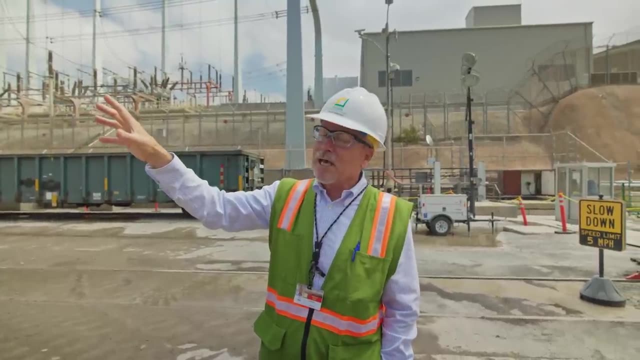 That's a termination point for tendons that stretched around the building. There's three buttresses like this 120 degrees apart. So once that building was tensioned it had the equivalent strength of about 12 feet of steel reinforced concrete. 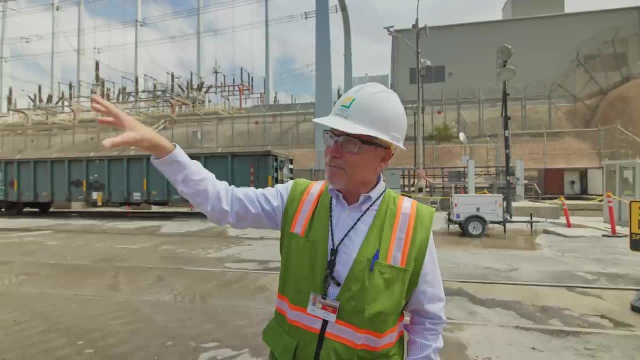 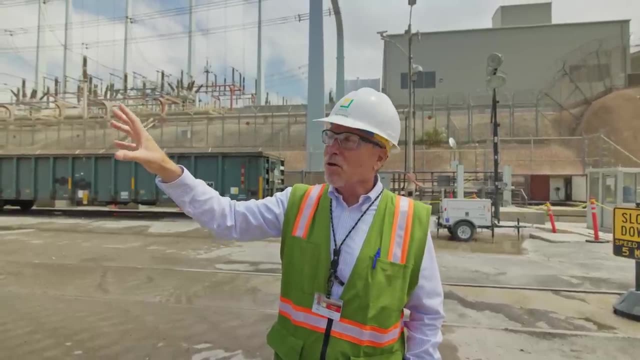 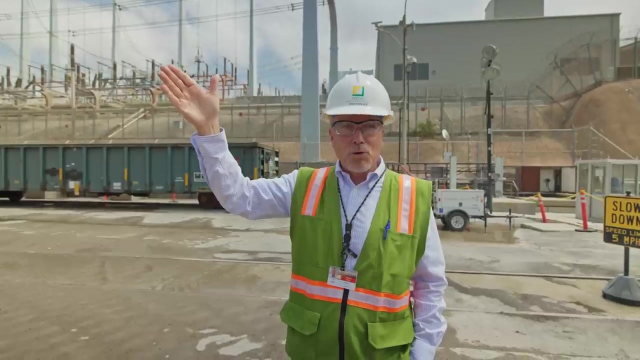 Substantial building. So why was it so substantial? Because inside the building was the nuclear steam supply system. It was operating at very high temperatures and pressures So there was a lot of energy in the reactor coolant system. In an unlikely scenario where there was like a loss of coolant accident. 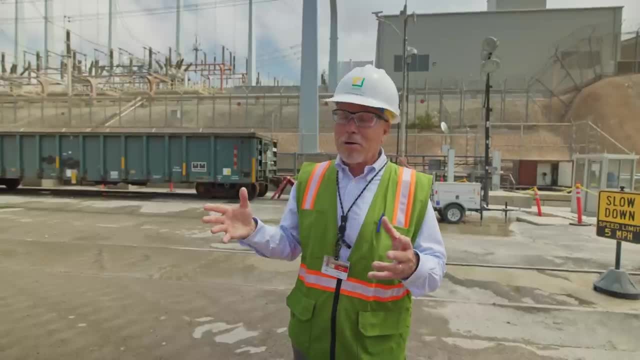 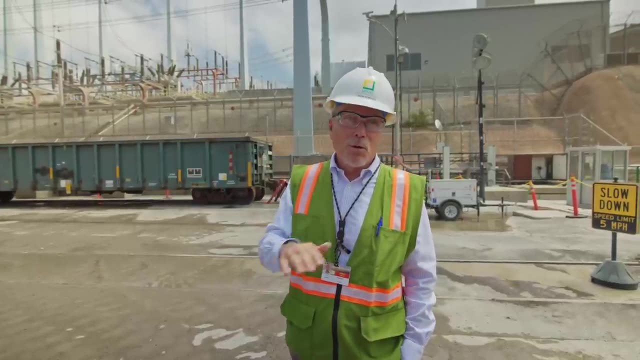 where we had a sudden break in the reactor coolant system and the water escapes would immediately turn to steam. you have a huge pressure event inside the building, going from around ambient up to about 60 psi, So this building was designed to withstand those types of events. 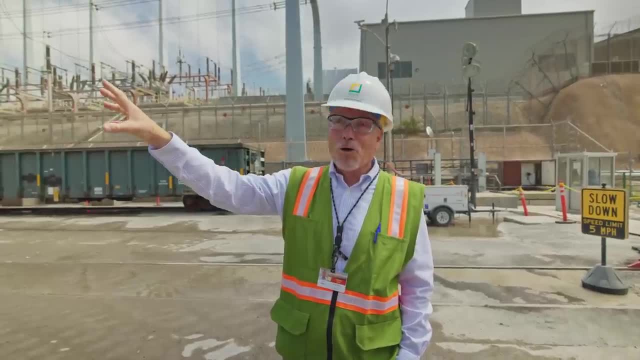 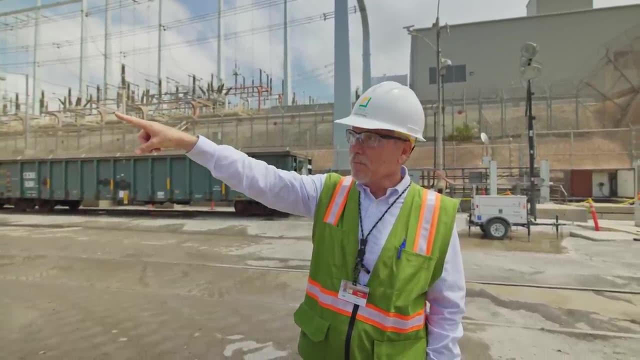 You know, you've heard of what happened at Chernobyl. Chernobyl didn't have a building like this. It was basically a tin structure. okay, Because they just had like a cover over the top of the reactor. It was like an industrial building, okay. 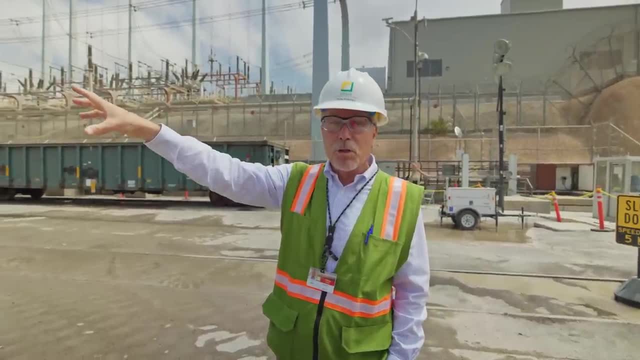 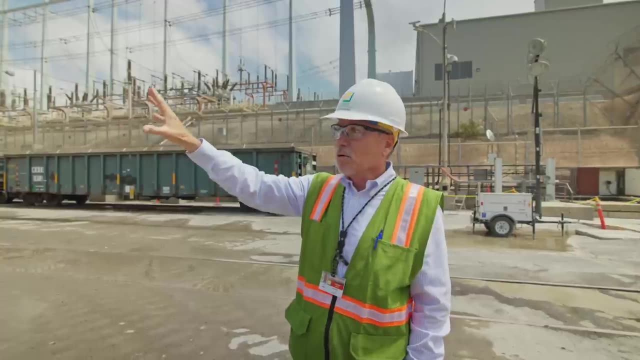 Unfortunately, And when things went wrong at Chernobyl, it didn't have a structure like this to protect the environment from the consequences of what's happening inside. So here we have a substantial building, lots of concrete, able to withstand the event. 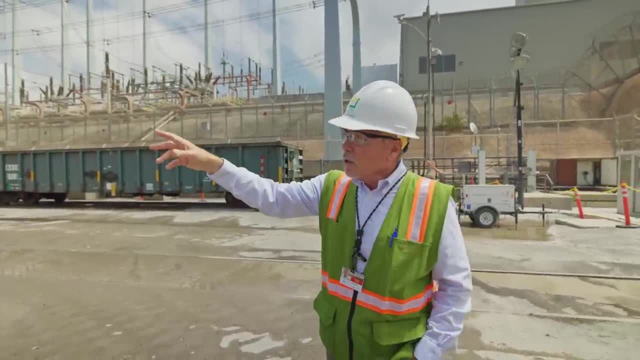 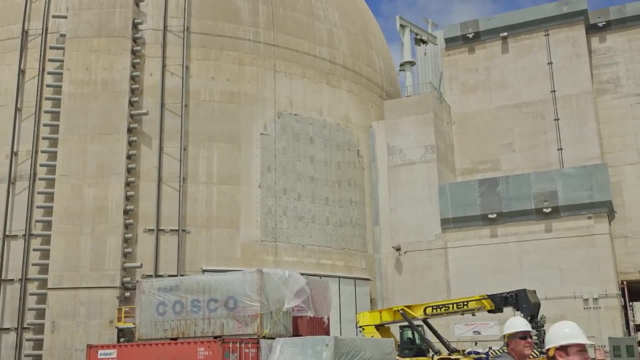 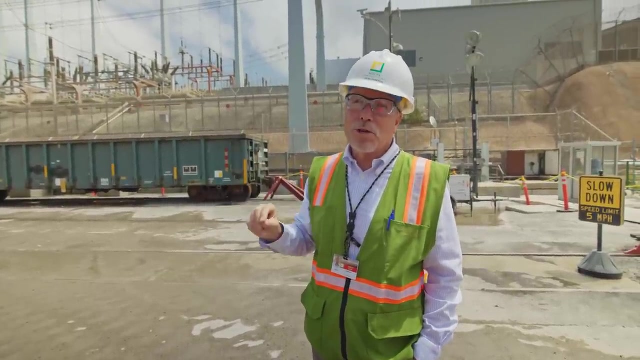 and it provides a lot of shielding too, okay. So you're asking: why do we have that place where we obviously made an opening Back in 2009 and 2010,. we replaced the steam generators in Units 2 and Units 3, okay. 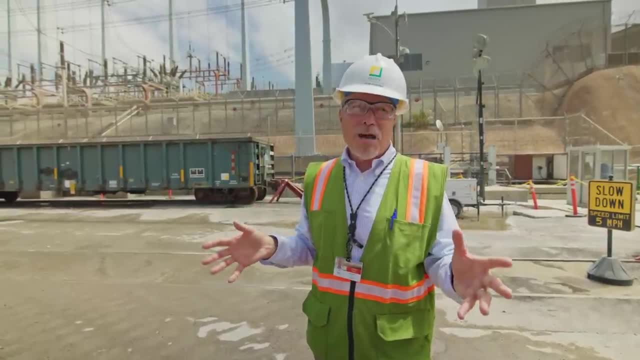 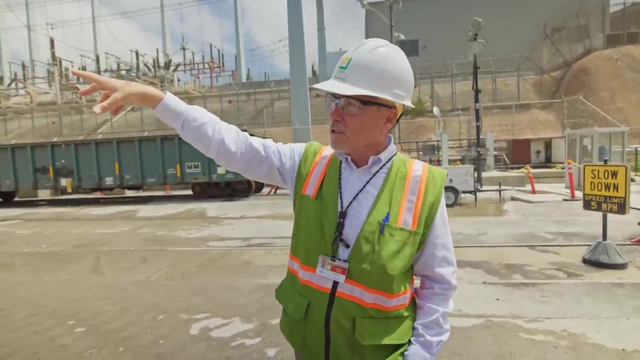 The steam generators are big components. They weigh about 550 tons. It was too big to fit through the equipment hatch, which was just below this area. So to support the process of replacing the old steam generators with new ones, we had to make this opening. 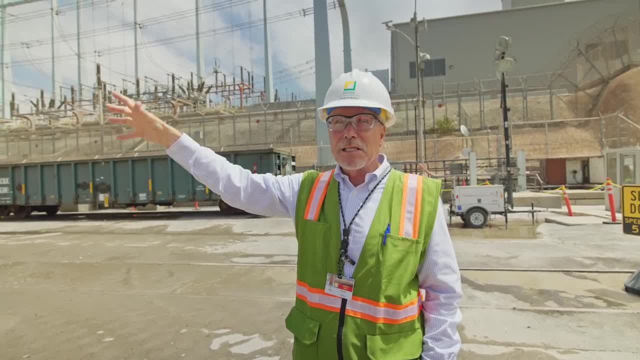 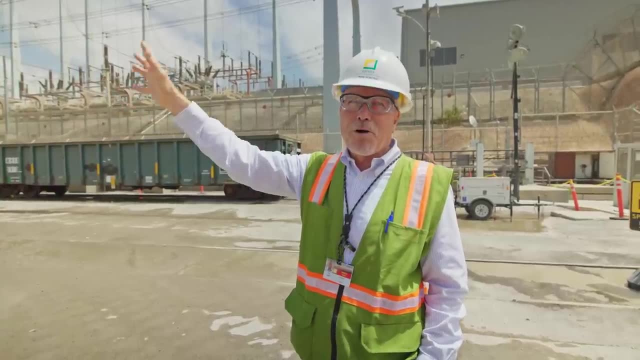 So to make the opening, we had to detension the building. remove the tendons, make the opening, replace the steam generators, then form this up, replace the rebar, place the concrete, let it cure and then we could re-tension the building. 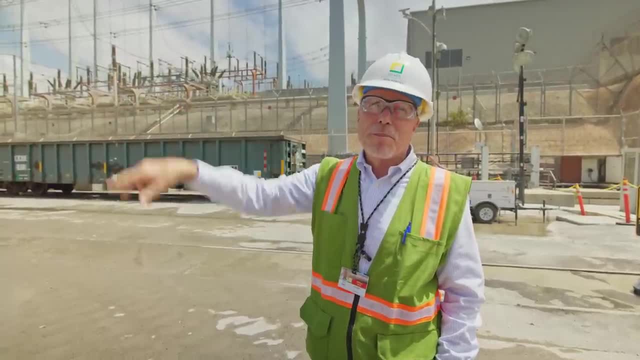 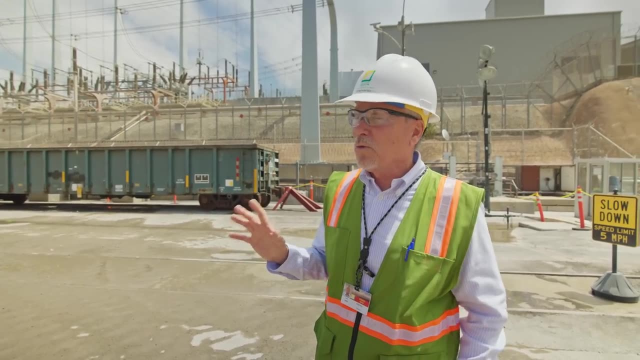 So that's why you see that scar, if you will up there. So how long did that whole process take? That took about 100 days per unit. Wow, Okay, With a very large force of people working here and a very super detailed schedule. 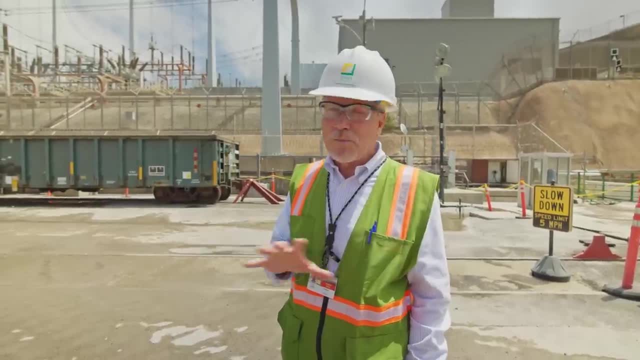 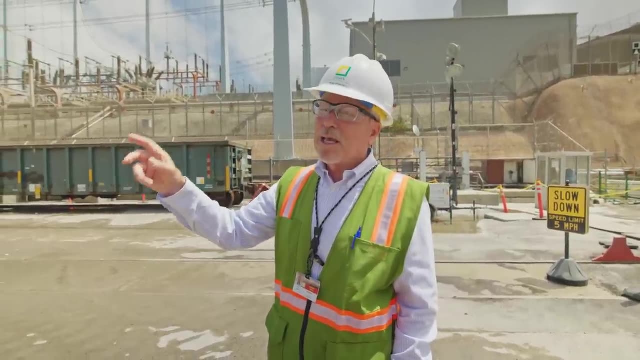 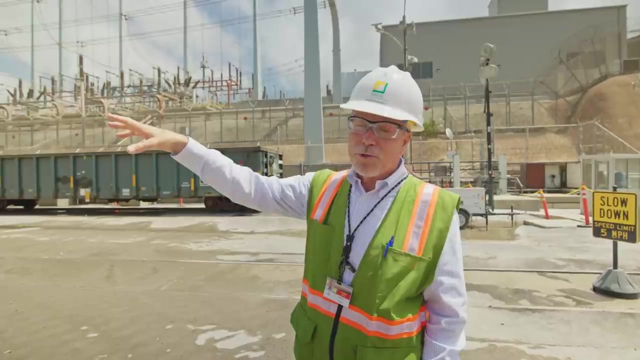 of many thousands of activities that had to be very carefully coordinated. It was quite a big project. That's why when we had the problem with these new steam generators- they're custom-made components. They've got about a five-year lead time And then you have to go through a replacement process like this. 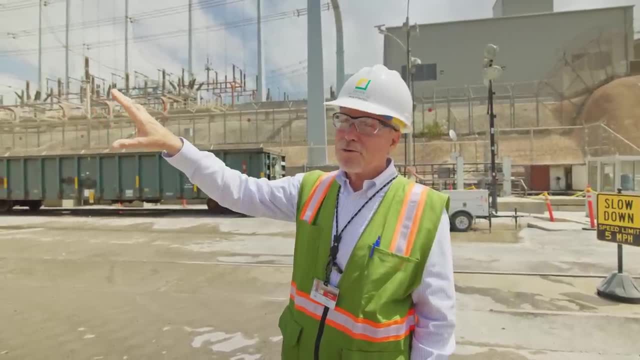 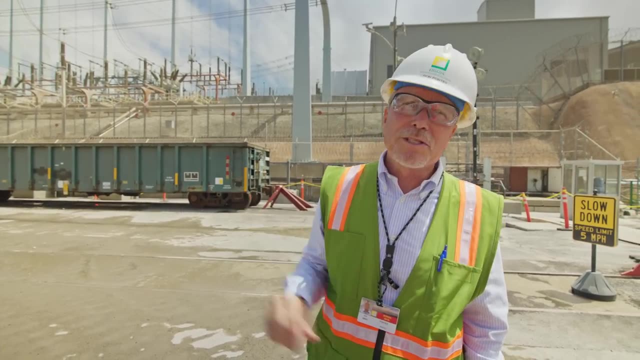 It became uneconomical for us. It became uneconomical for us to consider to keep the plant here and wait for new ones to show up to replace them, So that's why we decided to shut the plant. I'm curious, though, because that was right around the same time as 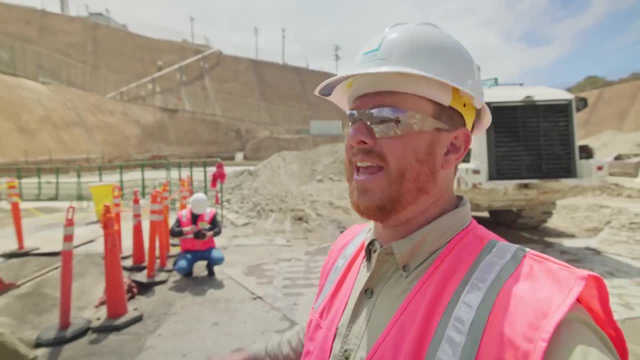 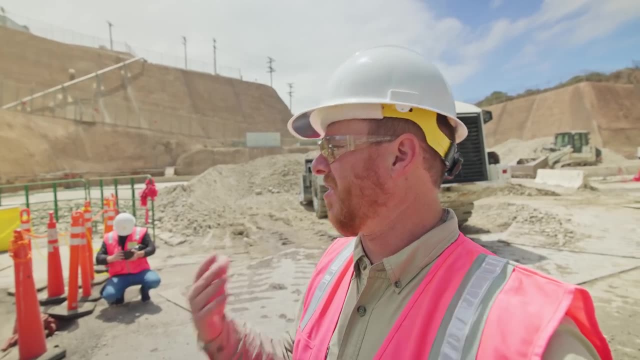 because what Fukushima was in 2011, right, 2011.. Yeah, And so I was always kind of curious: Was there just a ton of pressure from the community, from the local government, from all this other stuff also? 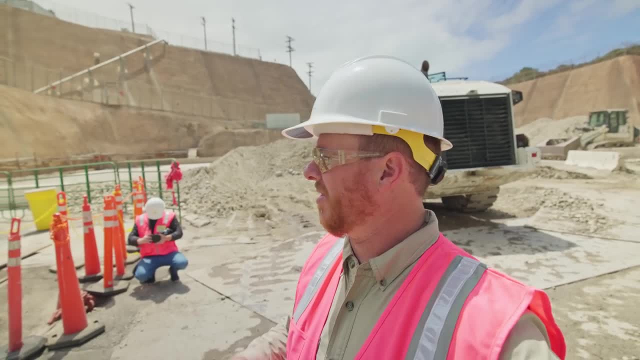 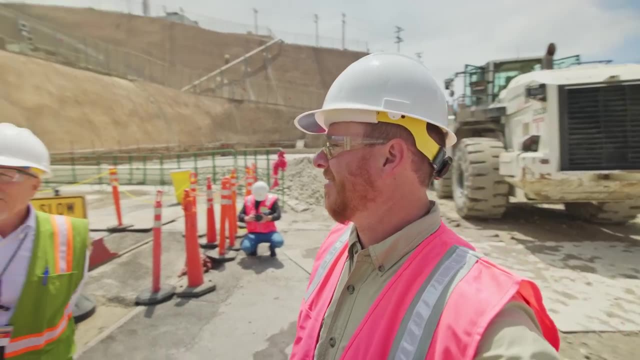 So Southern California Edison was just like you know what. fine, we'll listen to you guys. Since you guys are crying over this so much, we're just going to give you what you want. No, not really. Okay. What really transpired here was yes. 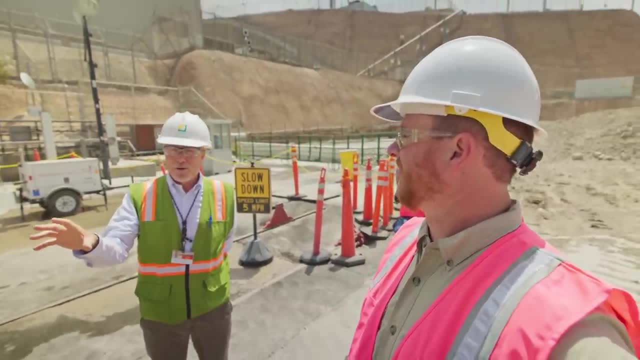 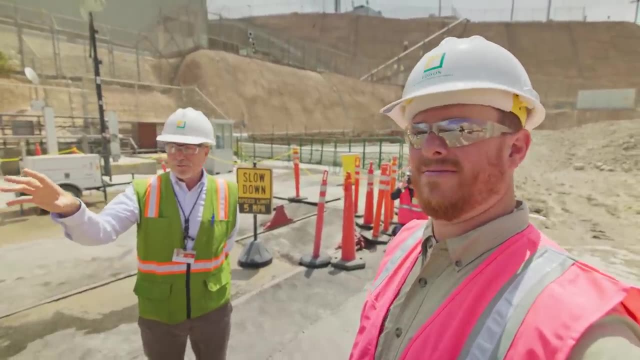 when we had the problems with the steam generators that occurred in 2012.. And as we investigated and understood better what had happened. yes, there was members of the public here that didn't want the plant to continue to operate, But they never wanted it here in the first place. 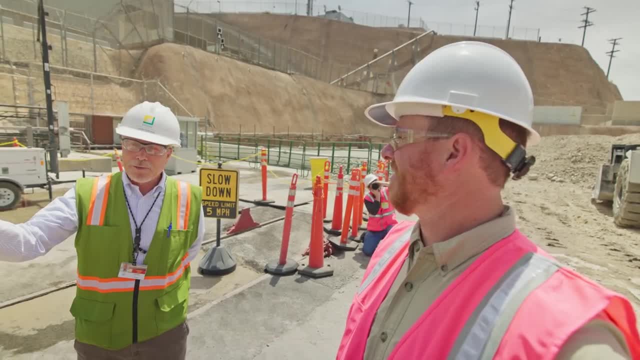 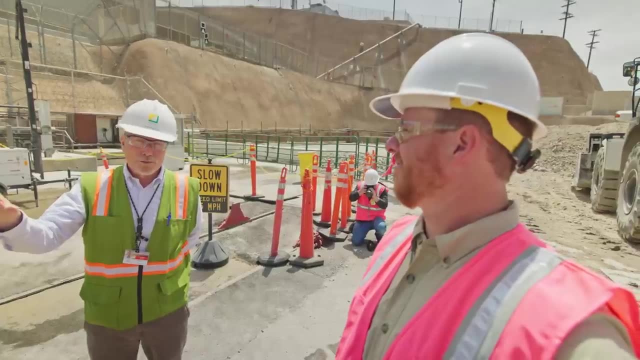 Some people didn't, But there were other people that were either ambivalent about it or were supportive. So you had a whole range of opinions. But there were people here that didn't want it, And that's absolutely true. But you know, from a technical perspective. 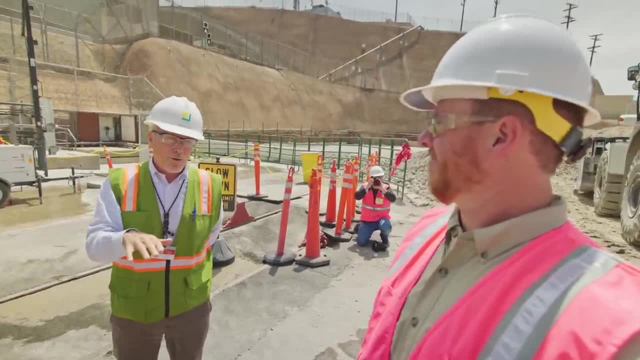 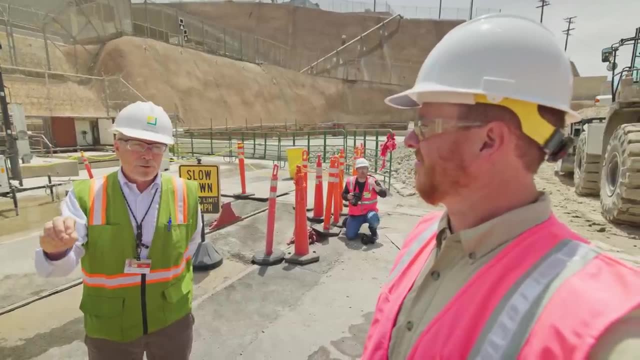 we felt that we could have restarted the plant and operated at a lower power level and continued to operate, But that convincing the regulator that we were able to do that became very hard and uncertain. So we finally just said it's better just to move on. 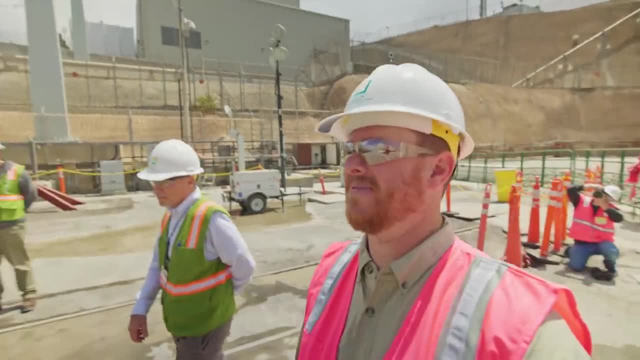 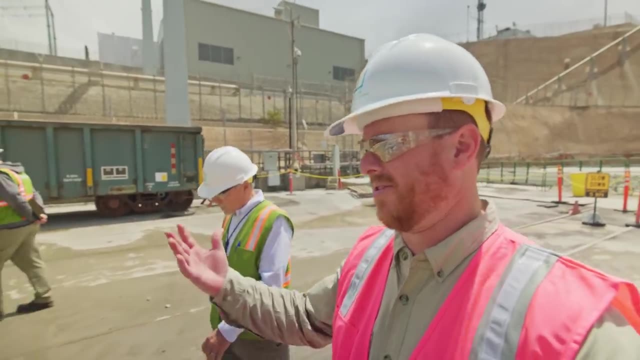 And that's what we did. Yeah, I just always was curious about that, because it was like such an interesting time period right there for nuclear energy, because everyone was like Germany was shutting down so many of their plants and all this stuff, And then this happened. 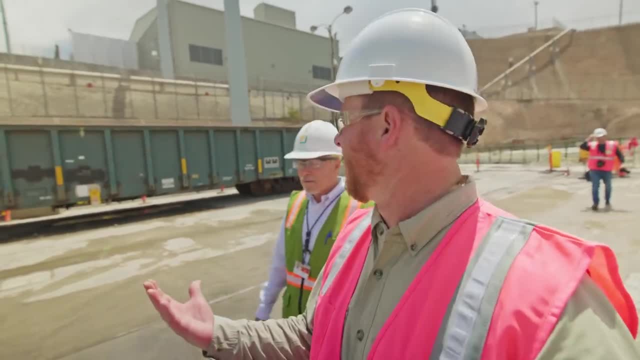 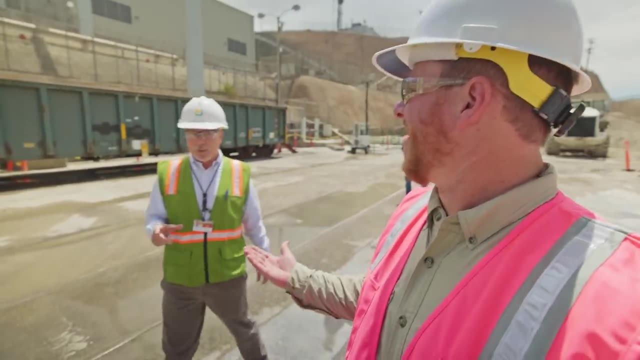 And I was just like: well, how much of this has to do with that? So you know it has to do with Fukushima. Fast forward to today and it's a different thought process about nuclear today, right Yeah, Especially in Western Europe right now. 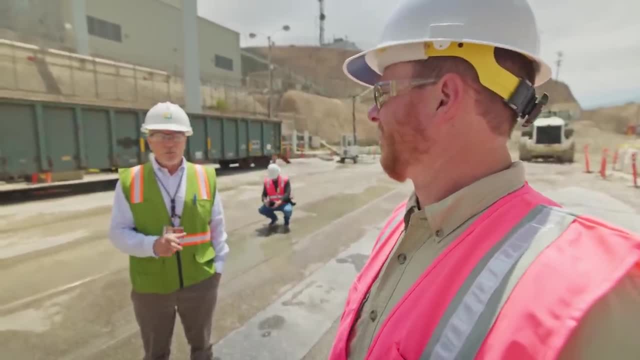 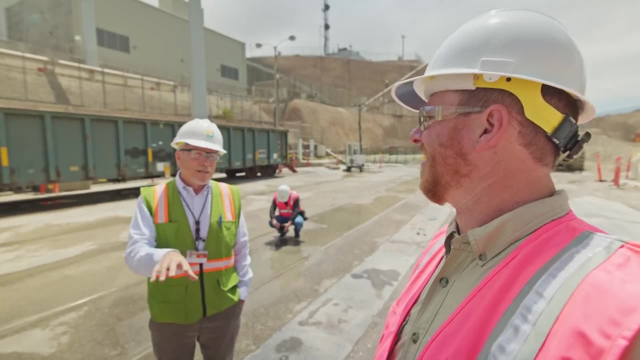 where there's a huge energy crunch right. Imagine if those nuclear plants were still available and operating today. What would be the? you know what would be the political issues around what's going on in Europe today. You know when you make these decisions. 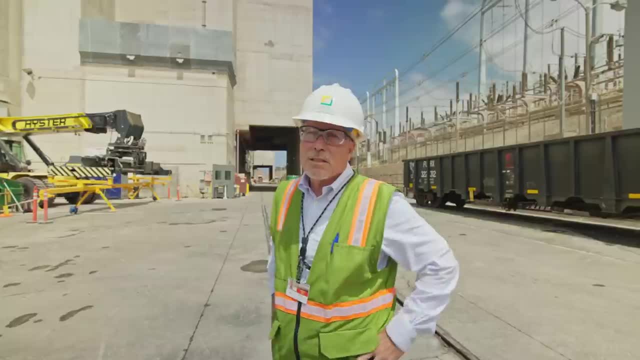 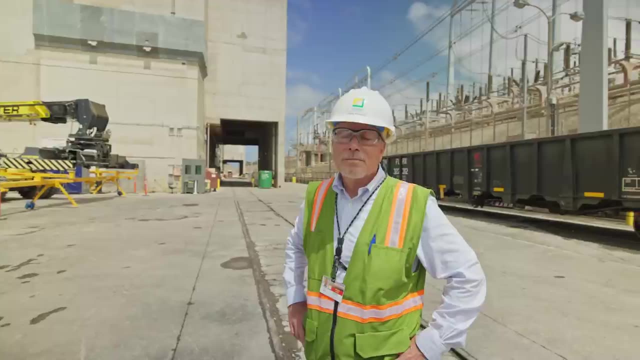 you don't know what the future holds either. So So now, how are they going to take down these vessels? Because, as I was understanding, they were going to do it from the bottom up, Correct? So how does that work? 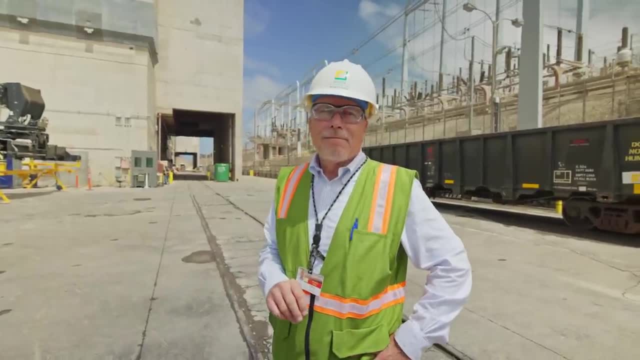 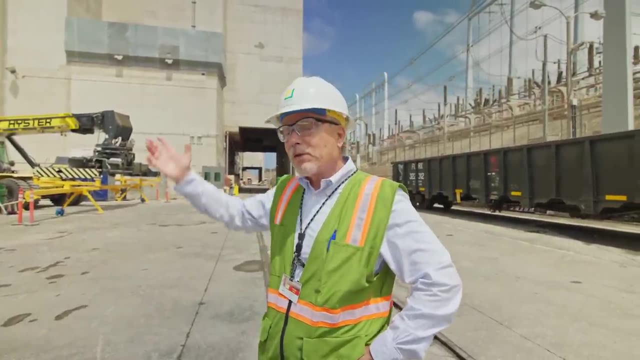 Yeah, that's pretty… Because that sounds engineerially challenging. Well, imagine what it would take if you try to do it from the top down. True, Okay, It'd be pretty hard to do and you'd have to manage all that material. 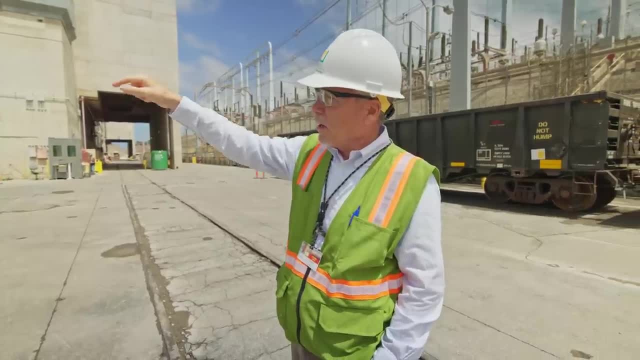 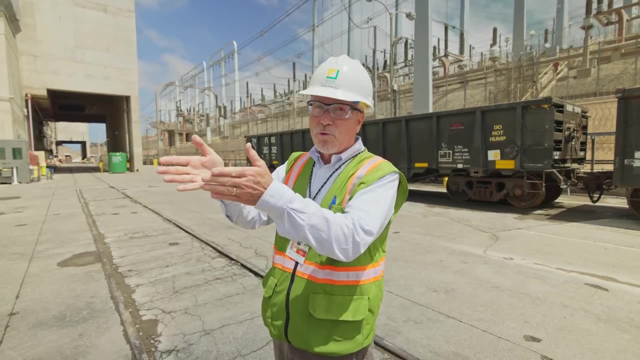 If you do it from the bottom, you basically just hammer at the building from the outside with those big excavators, and from the inside too, until you weaken this structure to a point where it just basically collapses. Okay, So just weaken the structure. and lifts of like six to eight feet or so. Give or take The building settles, muck out all the concrete and rebar, dispose of it and do it again. You do it over, and over and over again and eventually the building is gone. 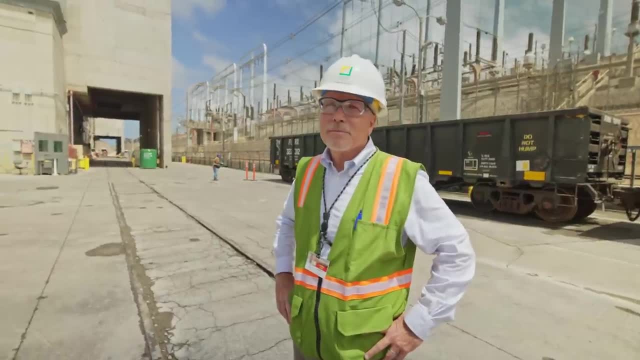 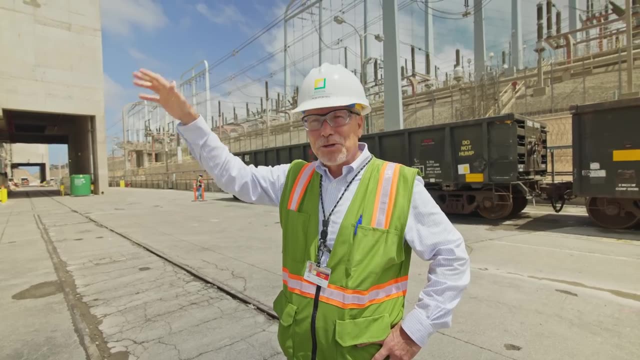 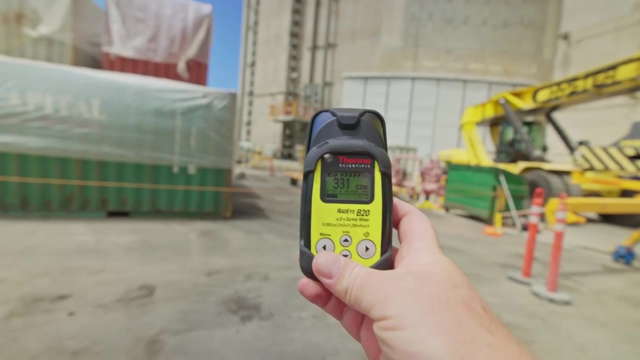 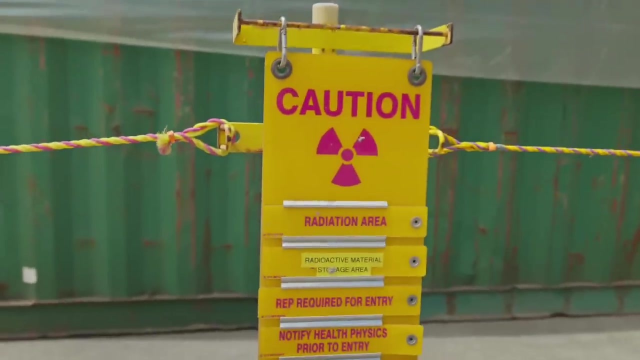 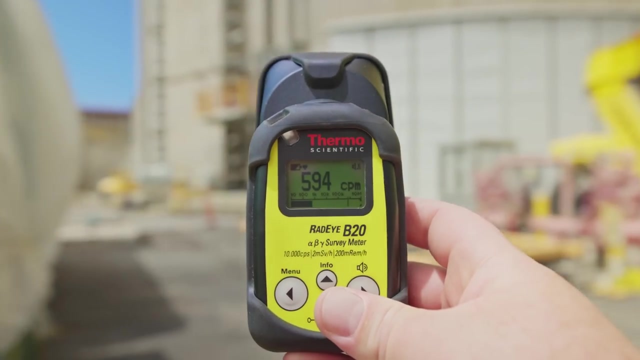 It's pretty cool actually. Now, how long would that take? How long is that process slated to take? I don't remember precisely, but it's in the neighborhood of about nine months to a year to remove the building. Wow, This level of around 800 counts per minute. 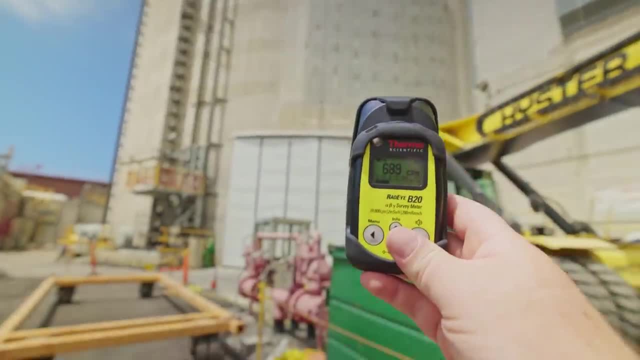 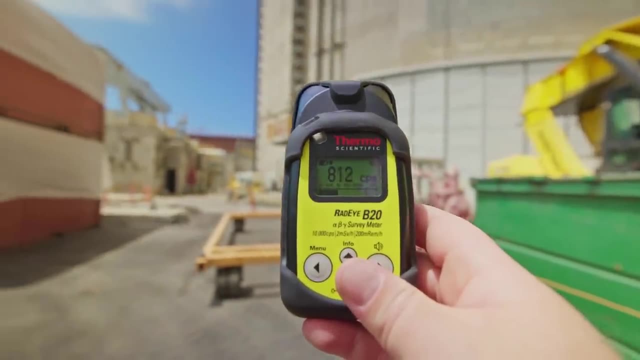 is about 20 times above background radiation, And the type of radiation that I'm more than likely detecting is from gamma radiation, based off the type of contaminants. that's here on the site. But now to put things into perspective, let's go to another location. 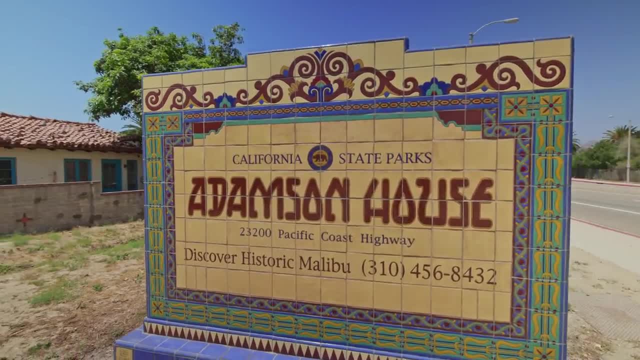 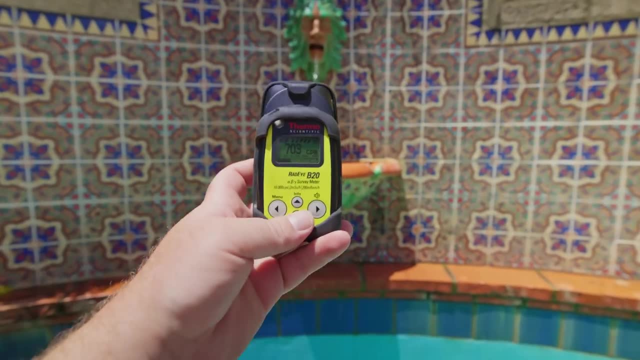 This is the Adamson House in Malibu, California, not too far away from San Onofre. I'm actually getting a higher level of radiation here at this fountain than what I was at San Onofre, And that's because these tiles actually contain uranium. 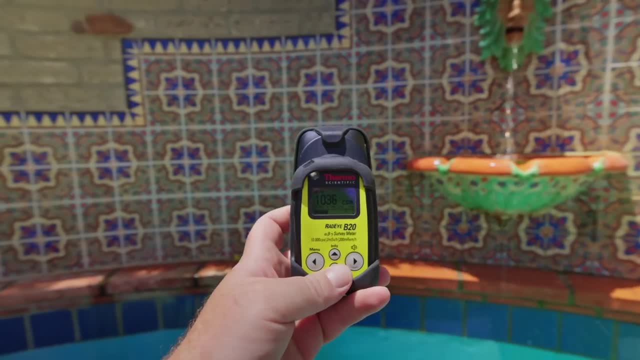 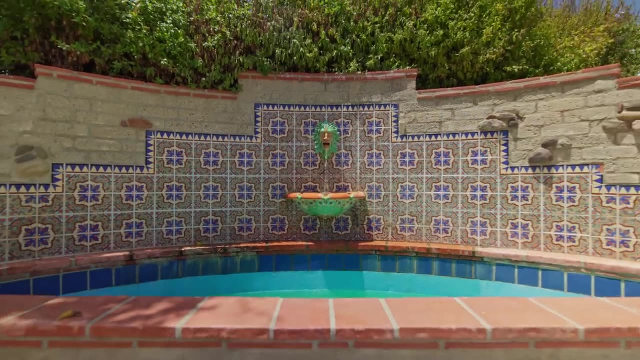 in the glazes which make them radioactive. Granted, the type of radiation that is coming off of these tiles is mainly beta radiation, whereas the type of radiation I was detecting at San Onofre was gamma radiation. So this building here, this is the fuel handling building. 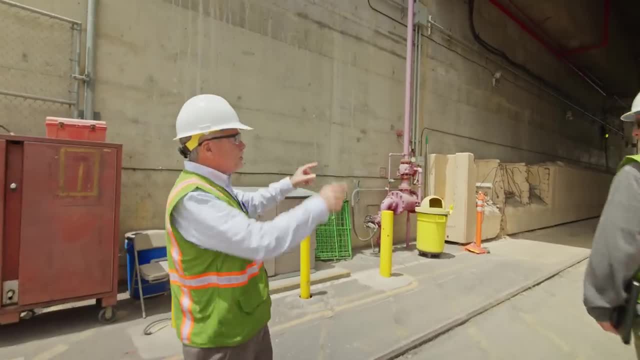 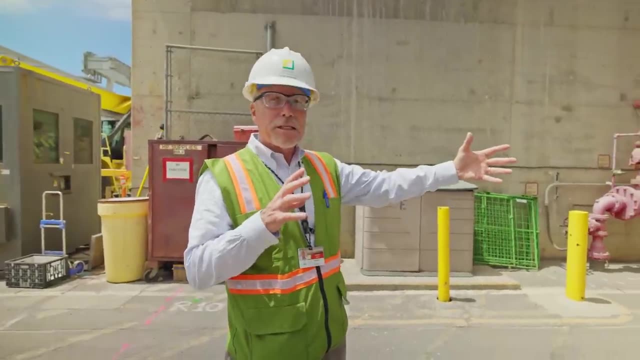 for Unit 3.. So this is a truck bay, this area. When new fuel arrived on site, it would come on a flatbed in specialized containers, okay, And then they would be. the containers would be lifted here through this small hatch. 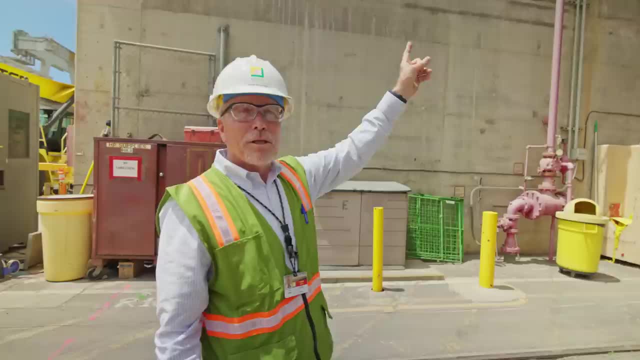 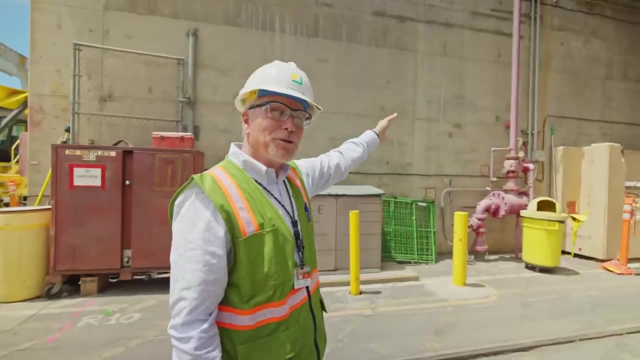 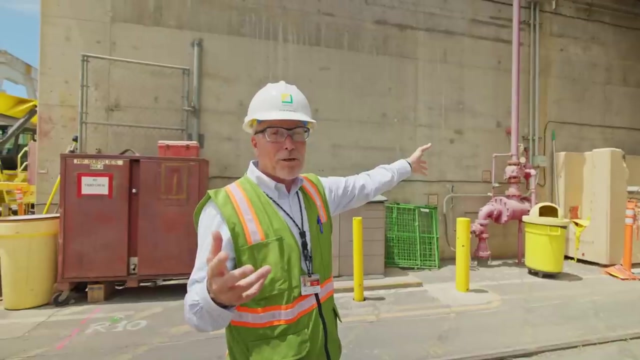 that hatch there into the fuel handling building. Fuel assemblies would be inspected and then placed in the fuel pool. okay, And then those new fuel assemblies would be used in the reactor and they would be used maybe three times for three cycles. So you know, assume three 18-month cycles. 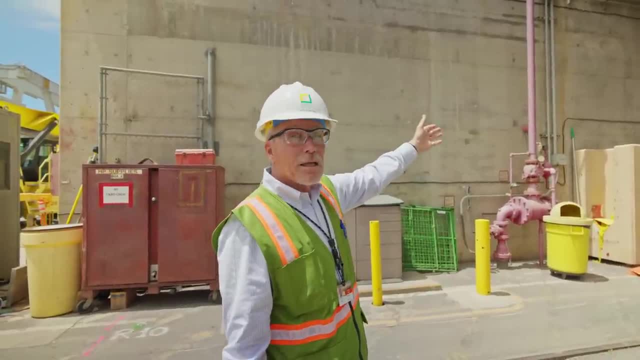 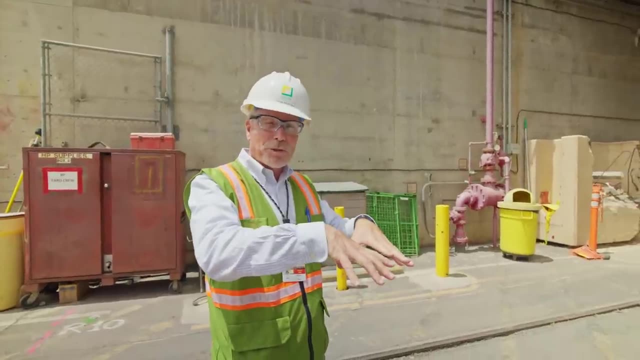 Wow, Typically two to three, So they just kind of rotate them where they are in the reactor. Yeah, they would move them around. They would change the core configuration every refueling outage, replenish it with some new fuel and discharge the old fuel that was used up. 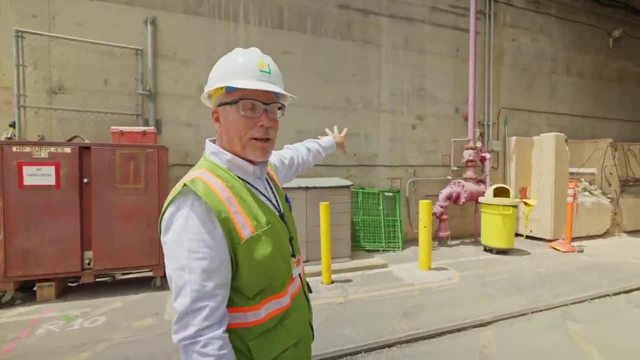 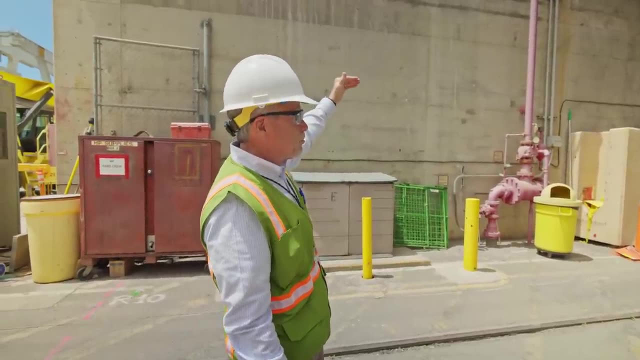 Okay, So then there's a refueling pool here in that side right, I just mentioned it. The pool, the top of that deck for the pool is about the 63-foot elevation- Again, 33 feet above us. It's full of water, demineralized water. 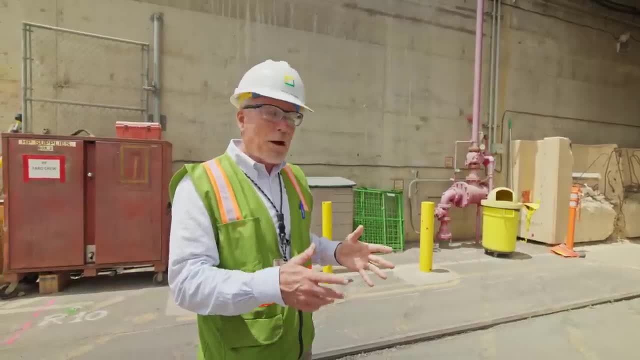 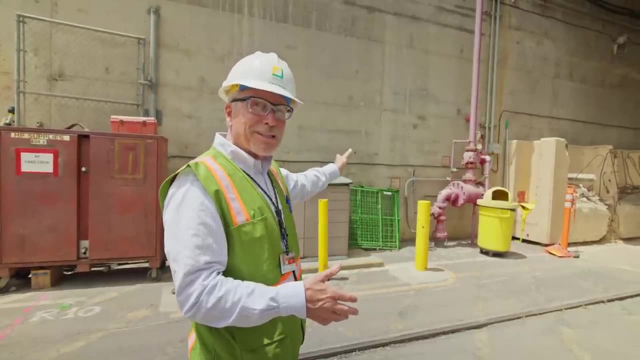 that kept the fuel cool while it was there, So that water was circulated through heat exchangers when we were operating through heat exchangers and the heat was eventually discharged to the ocean. The heat, not the water, Yeah, Okay. 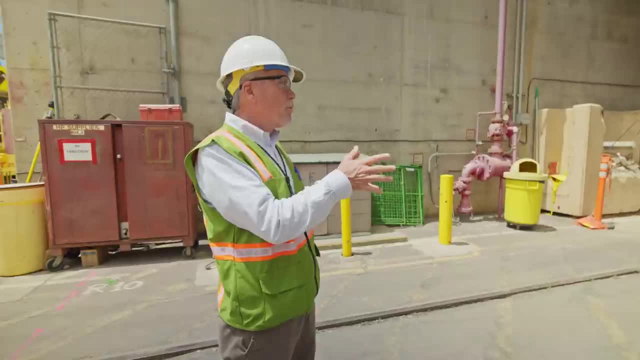 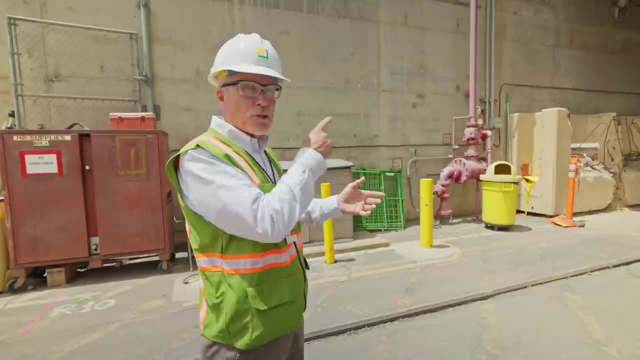 After we shut down the plant. they're not here anymore, but we installed some basically air conditioning units, big refrigeration units that were here, and we used those to cool the pool water until we could get all the fuel out. Okay, 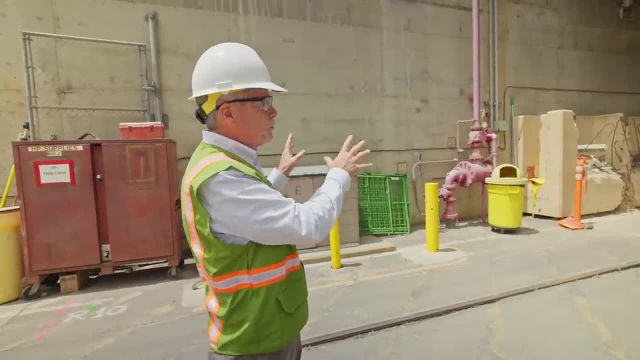 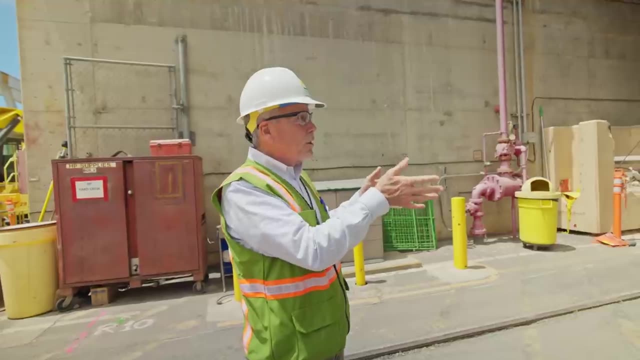 And the dry storage. Okay, So that's what this building was used for: housing new fuel and used fuel, and then what we call spent fuel, and then eventually, today, they're empty the fuel We've all just left in there. 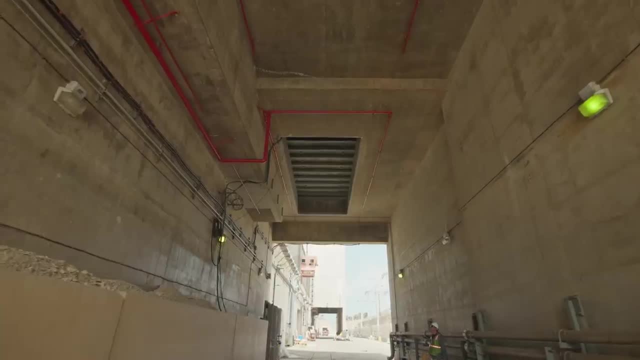 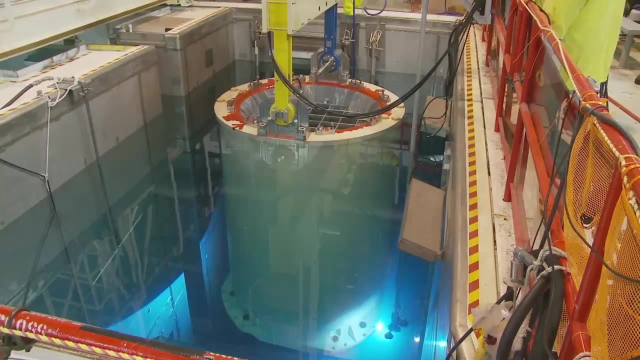 now it's water. That hatch is where the canisters of spent nuclear fuel, the dry storage canisters. they would be filled under water in this building. They'd be taken out of the pool. The water would be discharged from the canister. 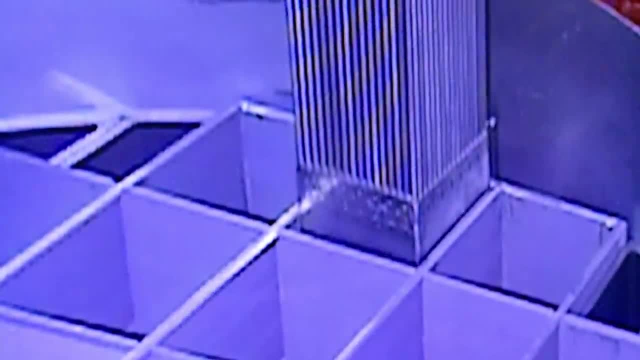 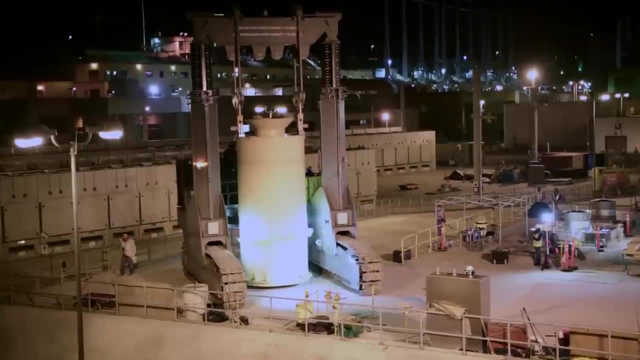 The canister will be dried. A lid like this, about nine inches thick, would be welded on the top of it. Then the canister would be handled through this hatch onto a wading transporter here and then hauled over to the dry storage. 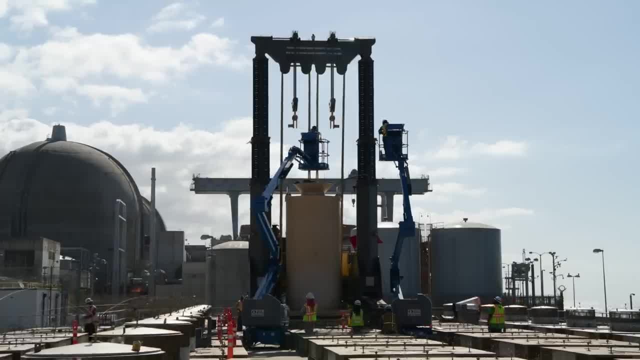 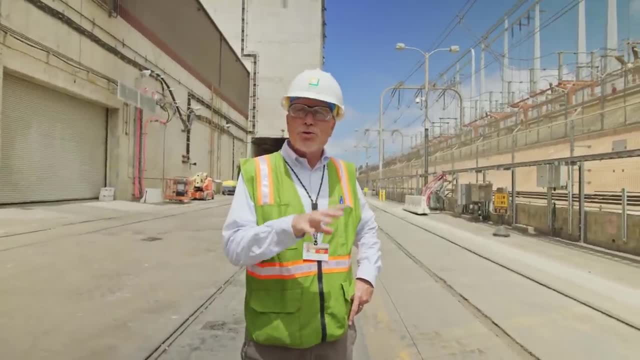 The dry storage facility, where it would be placed inside of a vault. Wow, We call this the restricted area. Okay, But it doesn't have any nuclear security attributes to it today. That's because all the spent nuclear fuel has been removed. 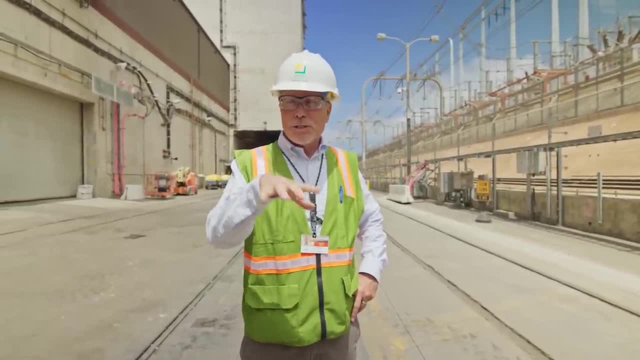 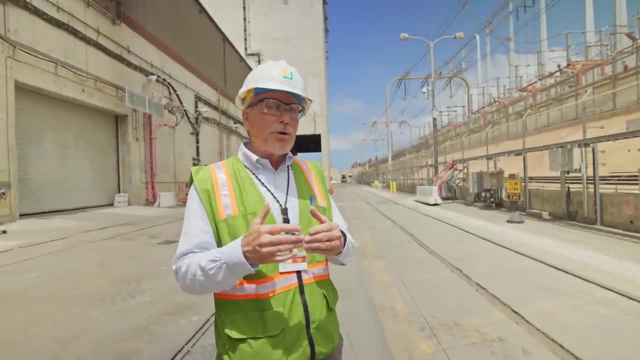 Okay, And after it was removed, we reduced this area to what we call a restricted area. Before then, when we had fuel here, it was called a protected area And the ability to get in here was very, very restricted and controlled. 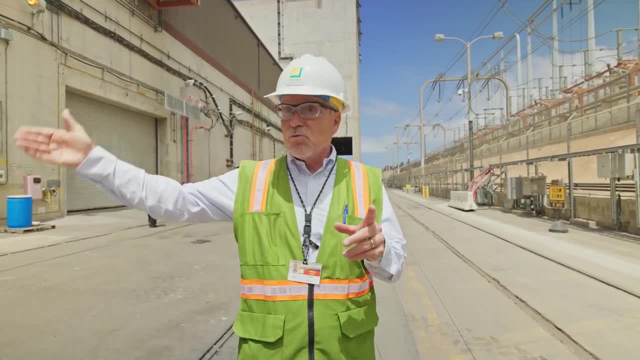 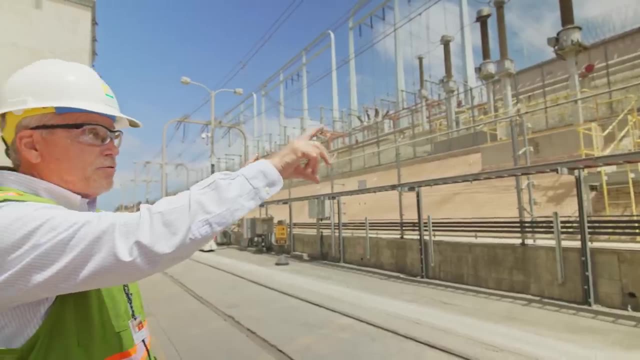 And the perimeter of this entire site and the seawall around here to the north side there was guarded by this fence, And this fence was an active fence. If you approached the fence it would alarm And there's camera systems no longer in use. 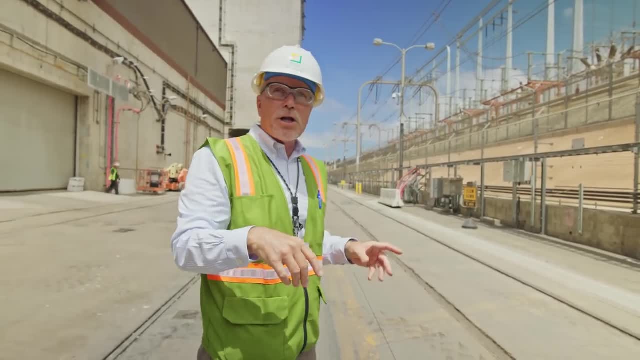 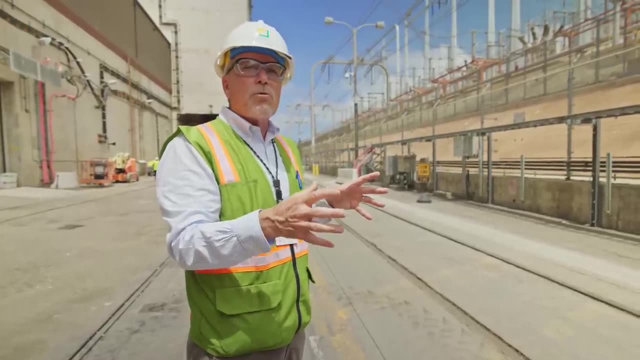 but you'll see cameras all over the place here that were monitored, looking for, you know, any potential intruders that would be trying to get into the plant. So the plant was very well guarded from a nuclear safety point of view when we were operating. 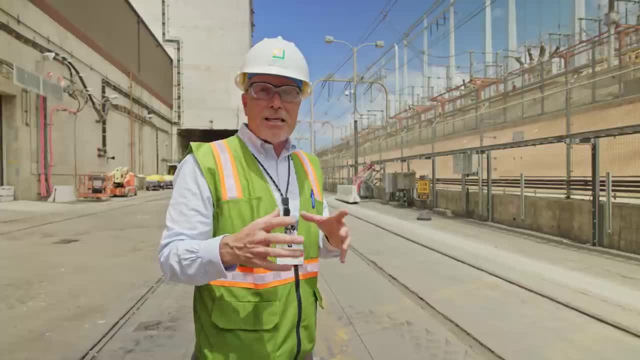 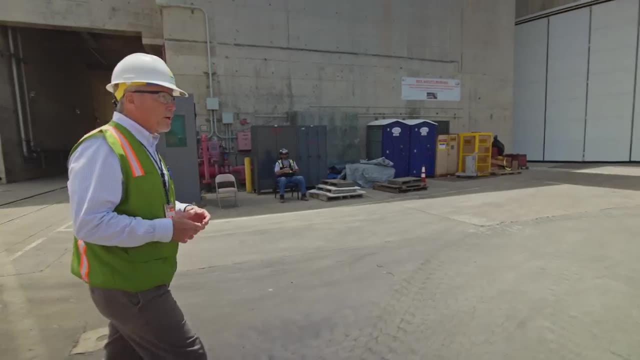 and while we had spent nuclear fuel here, Today the only protected area that remains for the plant is around the ispacy or dry storage facility, You know. if you want to take a radiation measurement, Oh yeah, I'd love to. 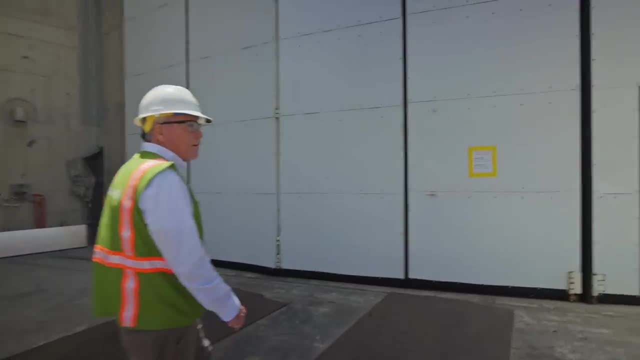 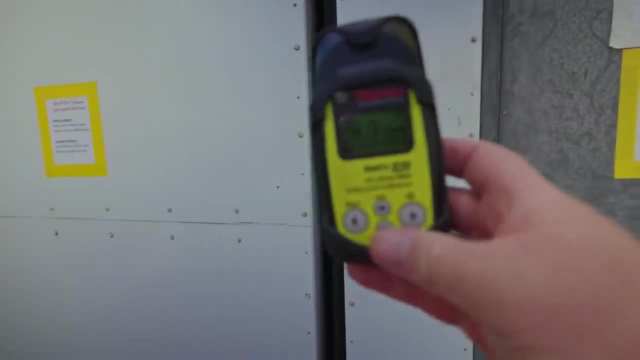 I hear something else. It sounds like a Ludlum in here. Oh there, it is Right there. I noticed that chirp. Nothing at all. Yeah, that's background. Yeah, Yeah, Now, if you were able to get past this. 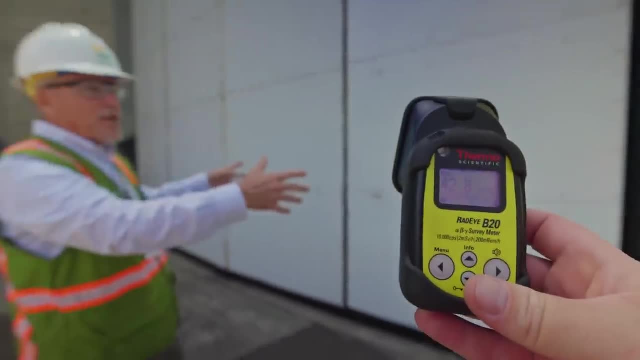 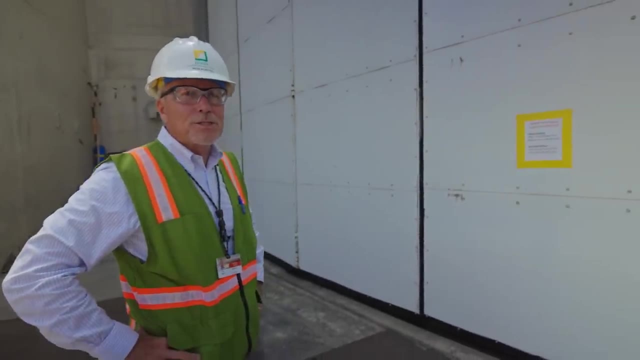 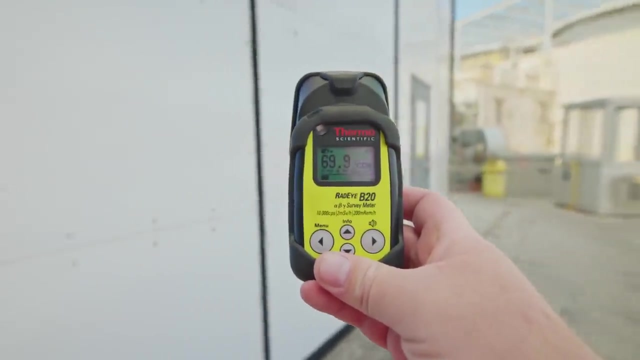 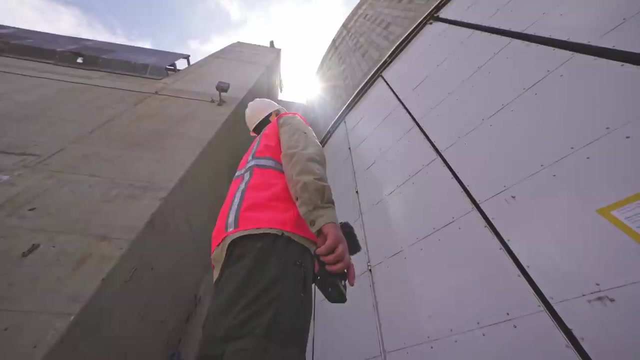 you can see inside, we've actually removed some of the internal bio-shield walls already, And even though those really thick structures are removed, you're not seeing any appreciable change in radiation out here. Since this video is getting a little long, 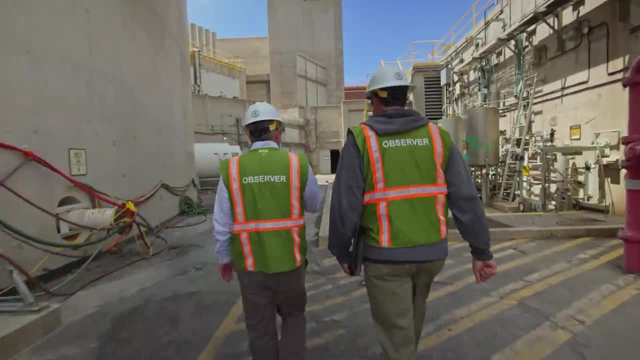 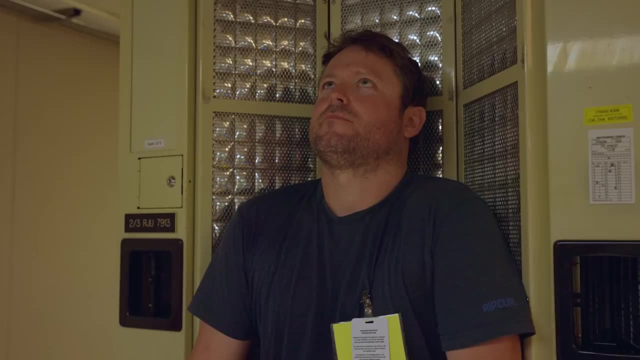 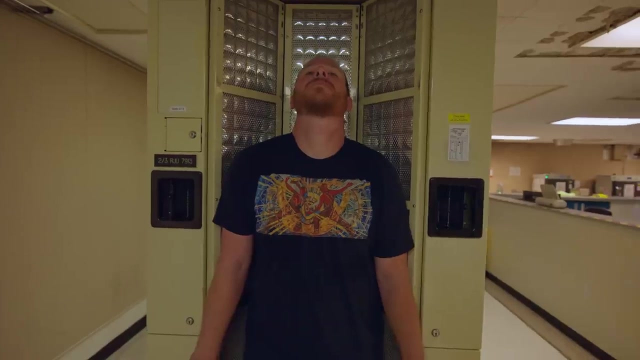 I'm going to split this trip into two parts. The second half is going to be dealing with the Radiological Controlled Area, or the RCA, where we get scanned a couple times, along with our camera gear, before entering and exiting. This is like the beginning of the Running Man. 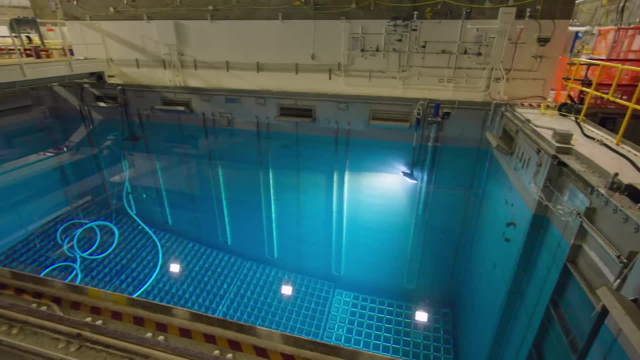 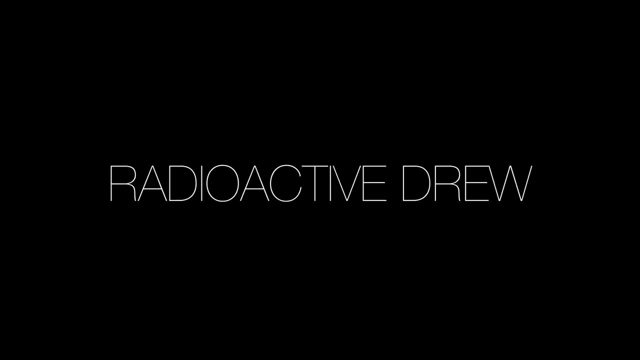 And in this area we get to see the spent fuel pool And then we get to take a trip out to see where the spent fuel now resides. So if you enjoyed this video, like it, subscribe and I'll see you in the next one. Captions by GetTranscribedcom.